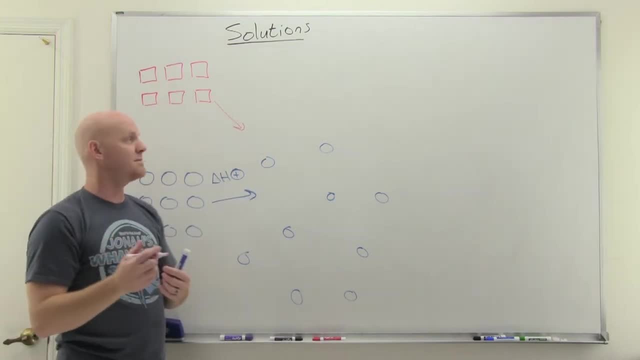 them out And any intermolecular forces holding them together have to overcome as well, And that is also going to have a positive delta H and be endothermic as well. However, then they're finally going to mix, And then they're going to mix, And then they're going to mix, And then they're going. 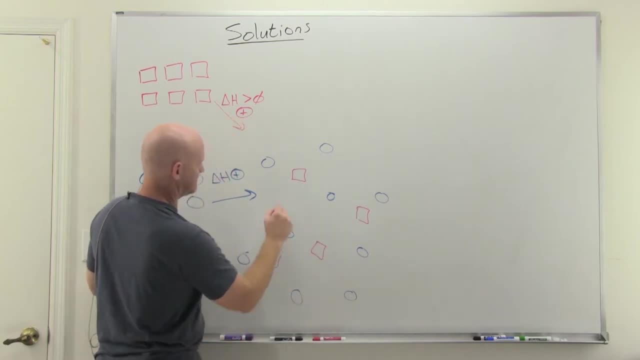 to mix. So, and again, we'll be spreading this out a little bit, So, but now they're going to mix, And once they mix, we are going to form some new interactions here. So, and these are going to be some new intermolecular forces, And what they are depends on the nature of the solute and the 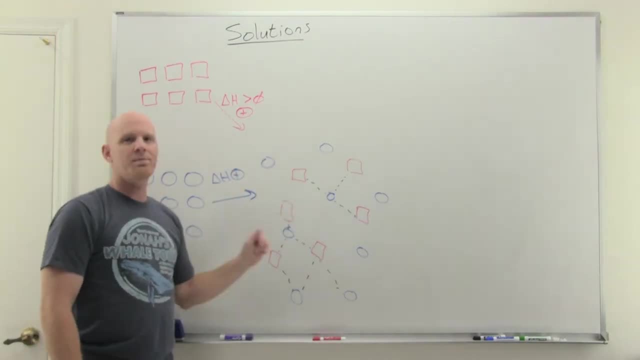 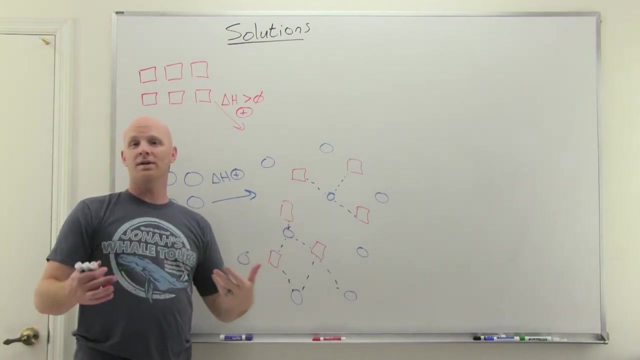 solvent and stuff, But we're going to form some of these new ones, And this is the only part of the solution process that's actually going to be exothermic. So, and again, we're going to be spreading this out a little bit. So, and again, we're going to be 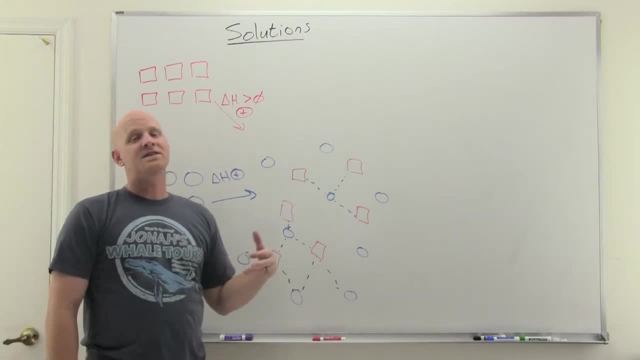 spreading this out a little bit, So, and again, we're going to be spreading this out a little bit, So we'll kind of see some examples here. So governing principle and solubility is that like dissolves like. So if the solute and solvent are alike in terms of polarity, then it's probably going to. 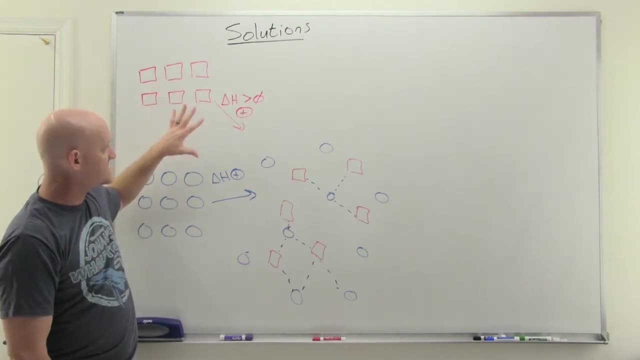 you know, the solute is probably going to dissolve in the solvent. So in this case, the reason for that is that, you know, let's say that, let's say this is water here, which has hydrogen bonding, the strongest intermolecular force, And let's say that this is methanol, which also has hydrogen. 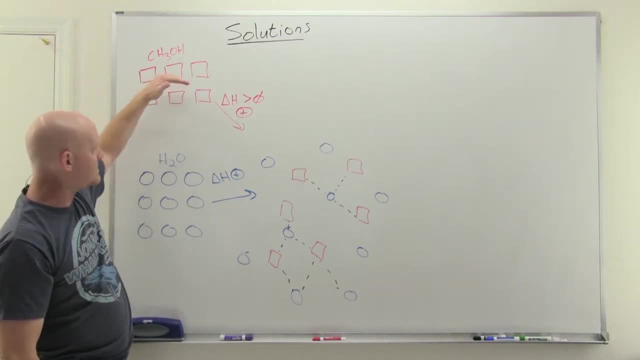 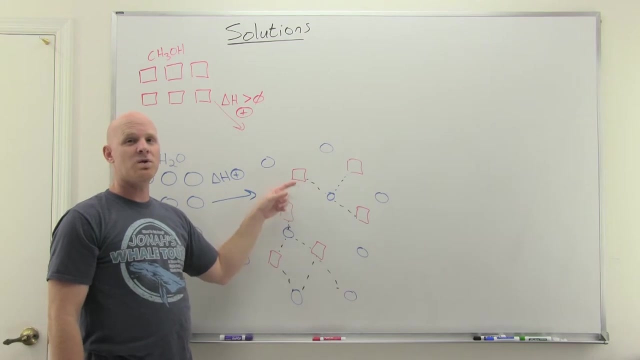 bonding for its strongest intermolecular force, And so it's rather strong forces. we've got to break apart to separate these, So it's pretty endothermic at the beginning, But the forces we're going to form between them at the end it's also going to be hydrogen bonding, And so the 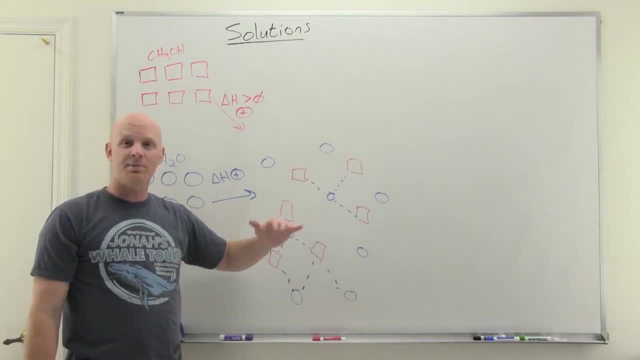 forces we create so, when they mix, are going to be roughly on par with the forces we had to break to separate them apart. And so, energetically, delta H for the entire process is probably not too far away from zero. So what ends up governing the process ends up being what we call. 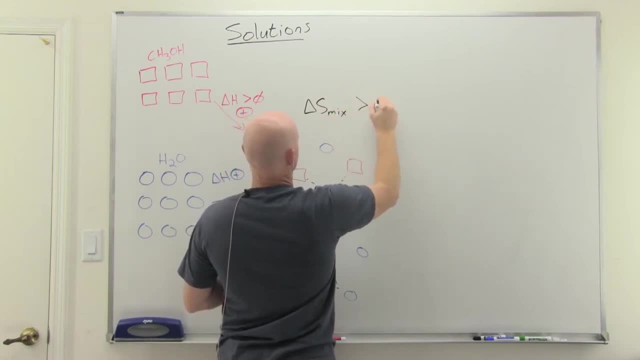 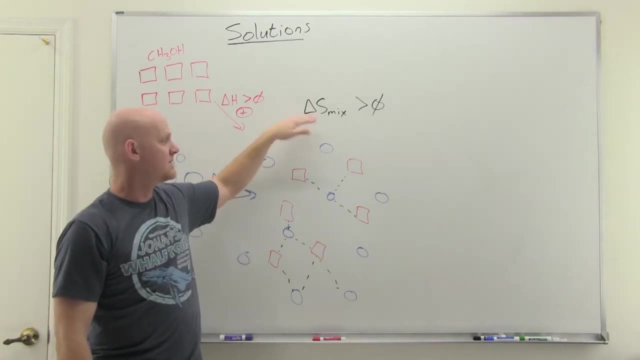 the delta S of mixing. So, and in this case, suffice to say you haven't really learned too much about what entropy is that's coming down the road in the future, But suffice to say it's related to disorder. So, and when you've got a mixture here, you've got more disorder than when 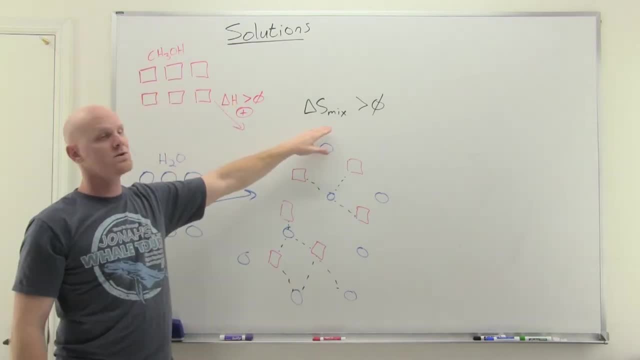 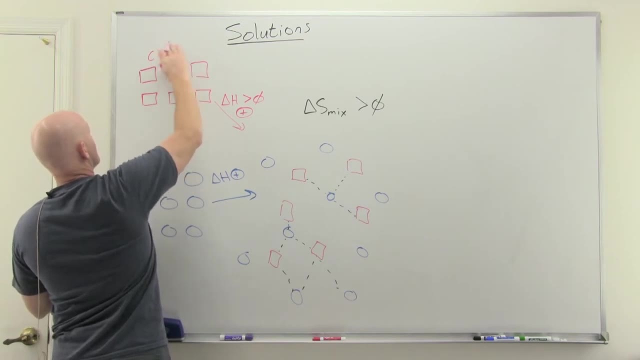 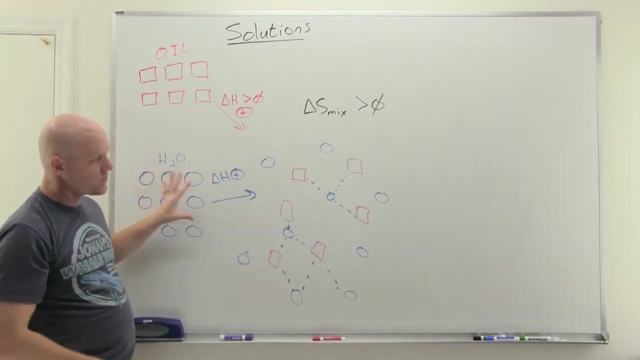 you had pure solute and pure solvent, And this is usually what's fueling things mixing. Now, if we contrast this for a second, let's say, instead of methanol up here, let's say we make this oil, And so these are now oil particles instead, And so again separating out the water. 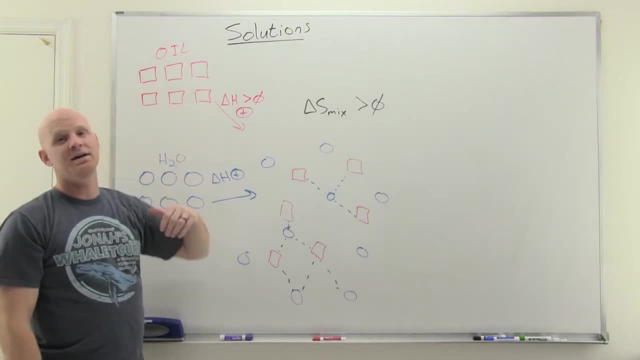 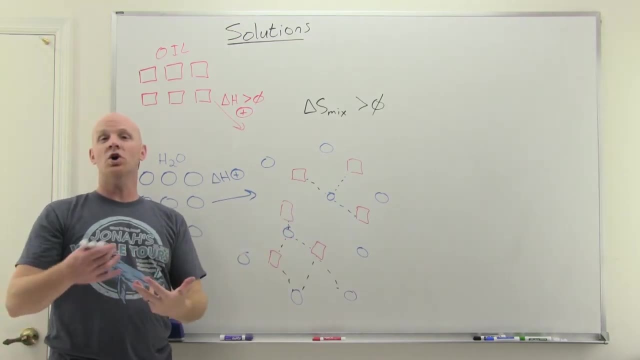 molecules is going to cost energy. Separating out the oil molecules is going to cost some energy as well. So, however, when they mix together to the degree that they do- and we know that oil and water largely don't mix- it doesn't mean they don't mix at all, but it means they mix very. 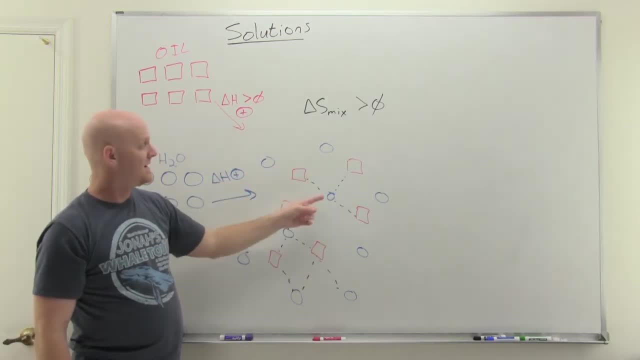 little, it turns out. So in the places where they did mix, it turns out these interactions were going to form between something very polar and something non-polar are not going to be very favorable, It turns out. So in fact, you'll find out that you know water's going to end up. forming highly ordered structures around the oil molecules that do make it in and stuff And it's a mess. but needless to say, it's a big energy expenditure to break these apart, especially if the hydrogen bonding and water but we don't form very strong interactions to replace them. 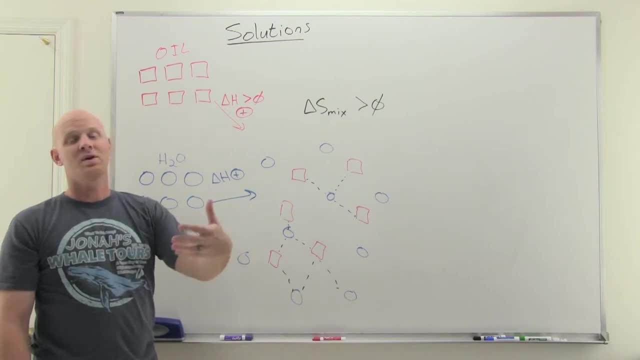 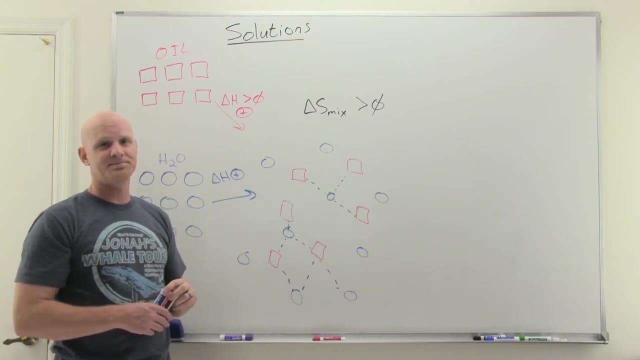 And so Delta H for the entire process now would be positive, which is not favorable for a spontaneous process, And it's not going to be spontaneous, and that's why oil and water don't mix. Cool. Now we've got just a little bit of vocab to talk about. We've got miscible and 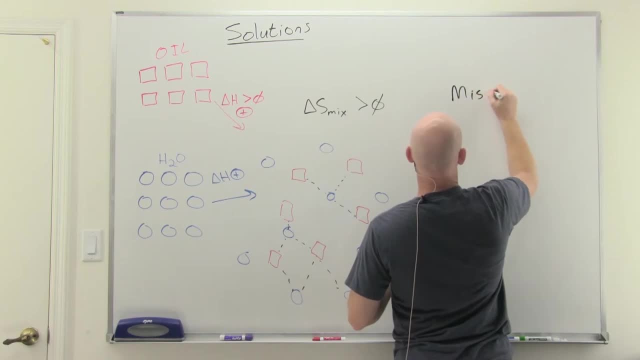 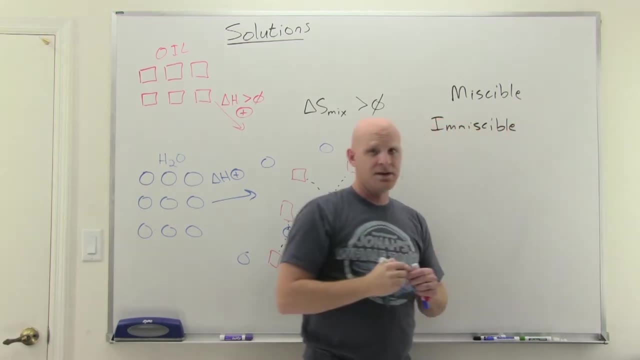 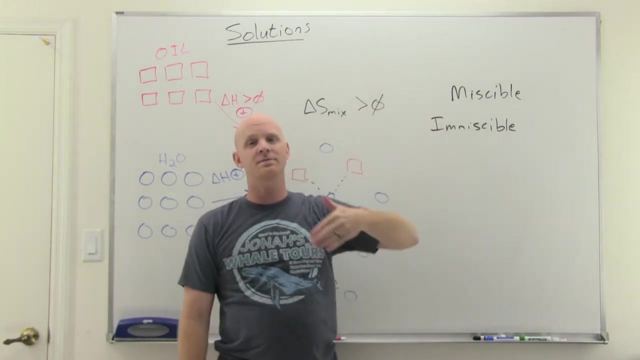 immiscible. Let's get those words up on the board here. So miscible and immiscible. So, and if you're mixing two liquids now, so if you're solutes, a liquid along with your solvent, so if they mix in any ratio, we refer to them as being miscible. And if they really don't mix and 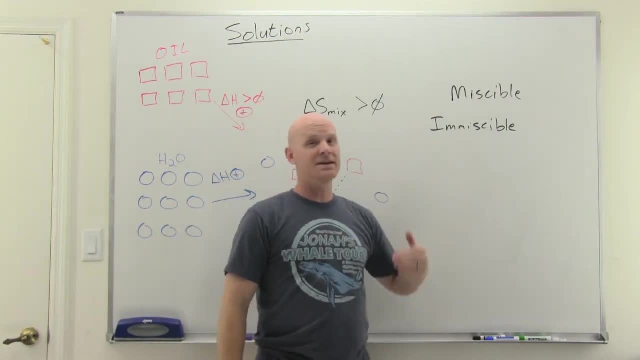 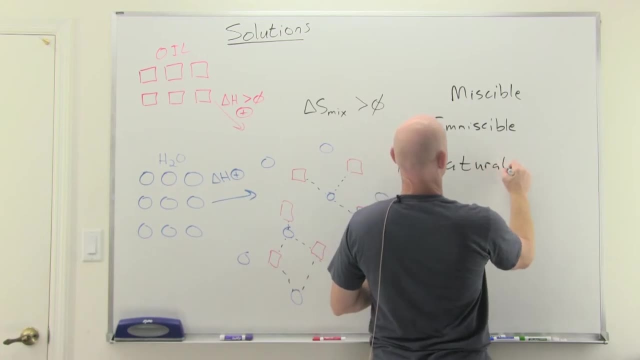 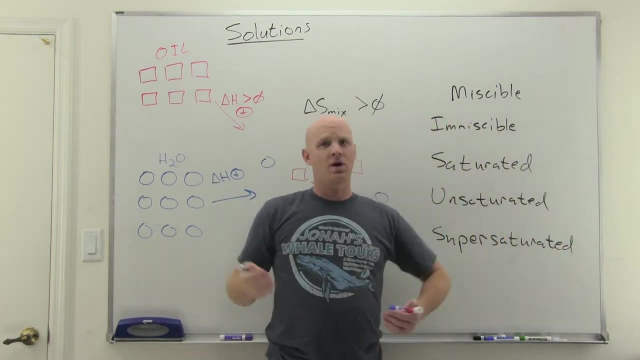 form two different layers, like oil and water, then we refer to them as being immiscible with each other. Uh, then we've got saturated, unsaturated and super saturated. So we'll start with unsaturated and saturated, And it turns out regardless of you know. 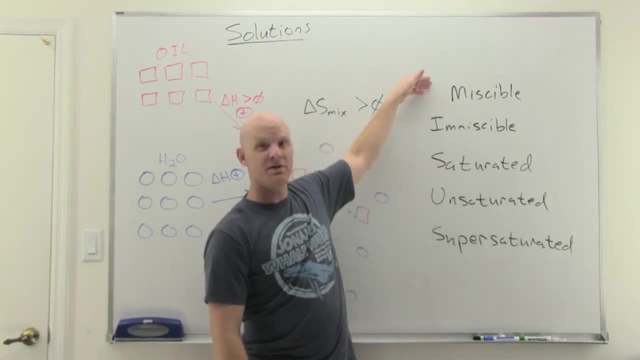 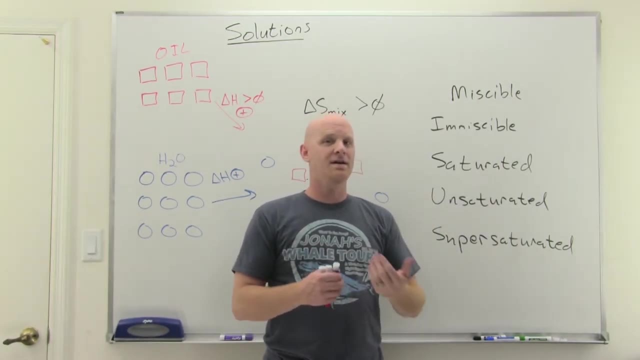 what your solvent and solute are. So outside of you know some miscible, immiscible, but for other solutes, typically you can only add so much into a solvent before you add any more than that, and it doesn't dissolve. And so once you've added the maximum you possibly, could we refer to that as 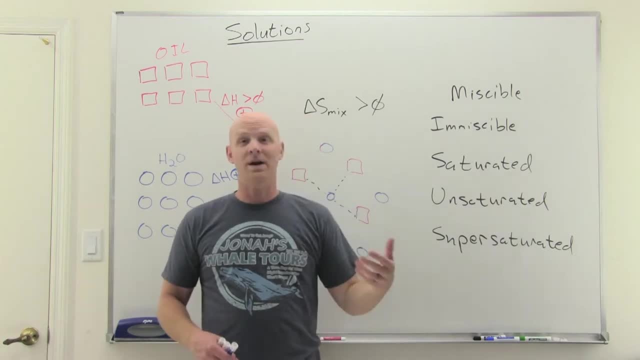 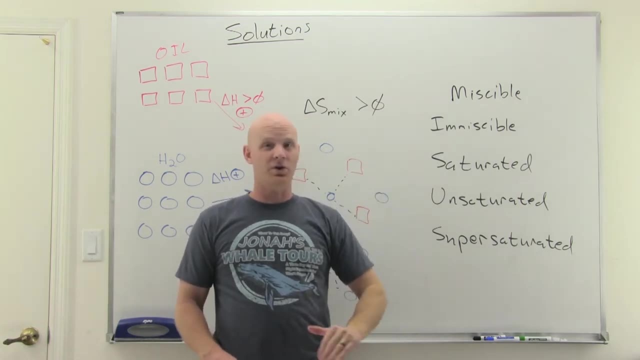 being saturated. Now we can add salt into water and you can add quite a bit of salt in the water, but you will eventually reach a point where you keep adding salt into water And all of a sudden you just get salt crystals that sink down to the bottom of your beaker or your pot or whatever. 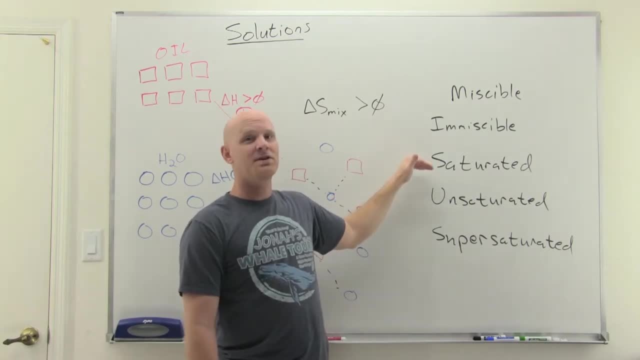 you're using. So, and at that point, when as much salt could be dissolved as is normally dissolved, we call it saturated, And up until that point, when we had less than that amount, we'd refer to that as an unsaturated solution. Cool, Then we can also talk about a super saturated. 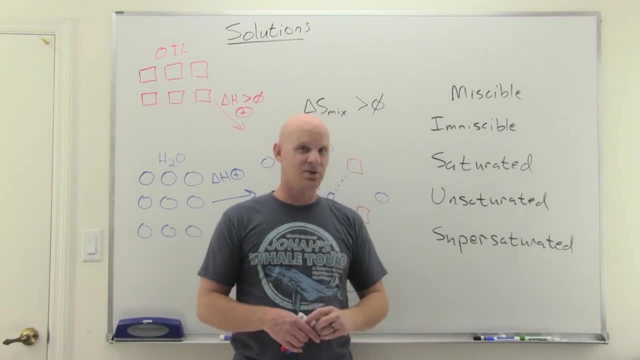 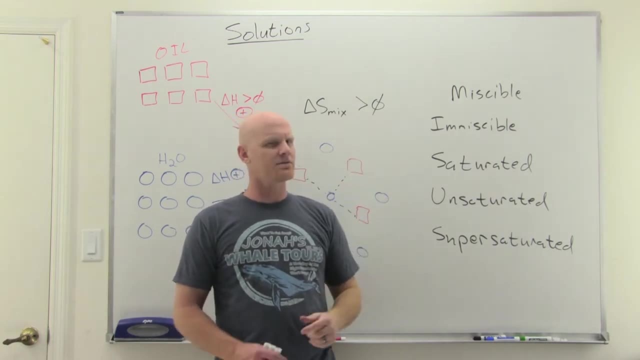 Solution. This is a kind of an anomaly here, So it's not a normal situation, but you can actually get more of a solute dissolved in some cases than the maximum, which seems kind of strange. So if you've ever made rock candy- and that's becoming less popular- 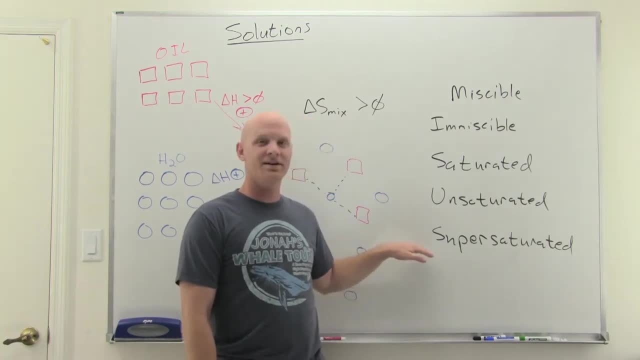 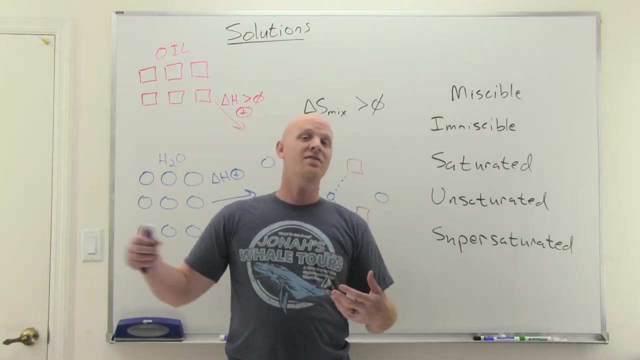 So. but if you grew up in my generation, you probably made rock candy somewhere along the way in school or preschool or something like that. And so to make rock candy, what they do is they heat up water, So usually to boiling, and then they add a bunch of sugar, And the reason you do it at very 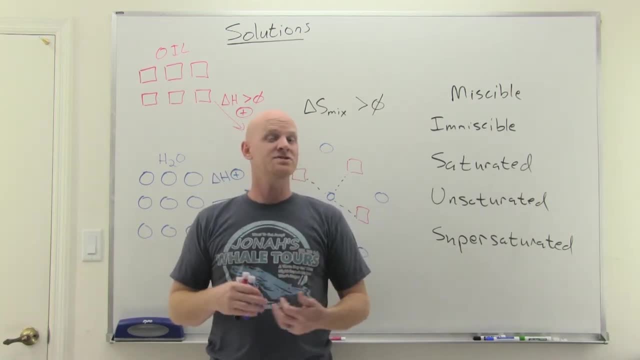 high temperature is because they're going to make rock candy. So they're going to make rock candy Temperatures, as you can dissolve a lot more sugar at high temperatures. thought more soluble it turns out, And we'll we'll see that in a trend in solubility here in a little bit. So, and if you, as long as you cool the water really slowly, so as it cools down, the solubility is going to go down And at some point you'll actually drop below. So you'll your temperature drop far enough that you'll drop below kind of the solubility of the amount of. 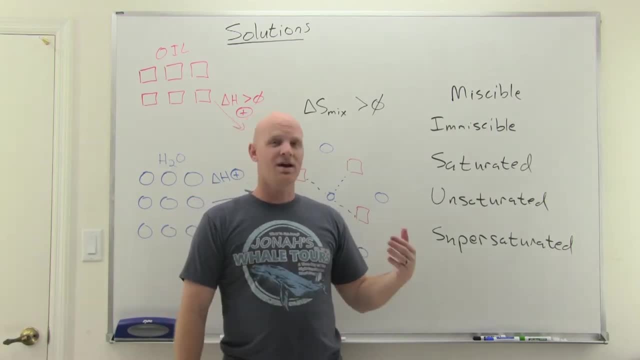 of sugar that's actually in your water when you're making this rock candy And so typically, if you just try to dissolve that much sugar into that water at that lower temperature now you wouldn't be able to do it. but in this creative way where we've heated it up and very 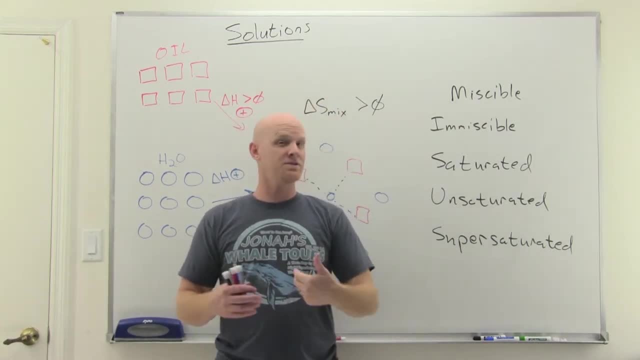 slowly cooled it down, you've ended up with an unstable situation where you've got more sugar dissolved in the water than would normally be able to stay in the water, And it turns out it's not a stable situation. So and if you drop a crystal of sugar in there or if you put something with 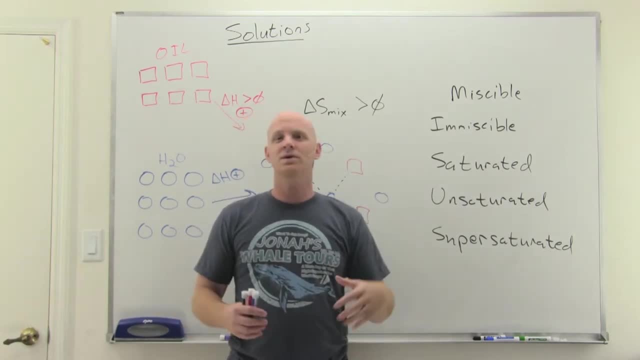 jagged edges like a piece of string or a stick or you know things of this sort you're giving, So you're giving a seed, if you will, for the crystals to grow on And all of a sudden you 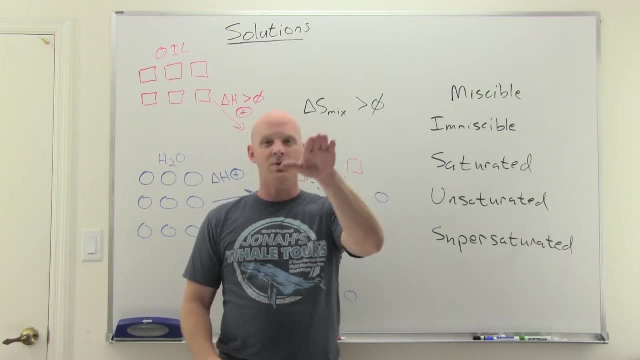 just get crystals everywhere and crystals come out of that solution. Until we get to the point where- until we go back to having just a plain old saturated solution. So super saturates when you have more again solute than the normal maximum dissolved but again it's an unstable. 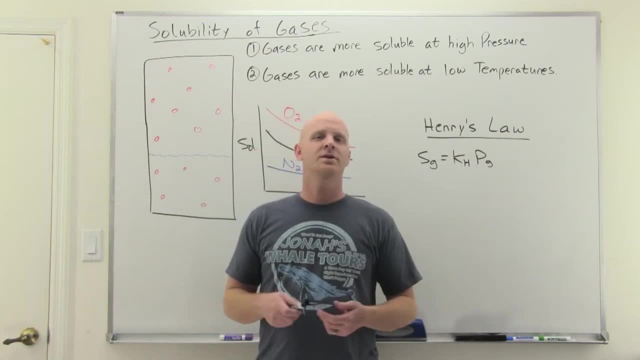 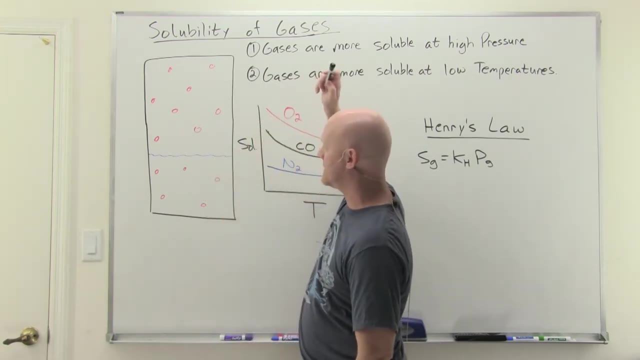 and an abnormal situation. Next one: I'll take a look at the solubility of first gases in different solvents and then solids in different solvents, And we'll start with the gases here. and turns out the solubility of a gas in a liquid and it seems a little bit counterintuitive. but 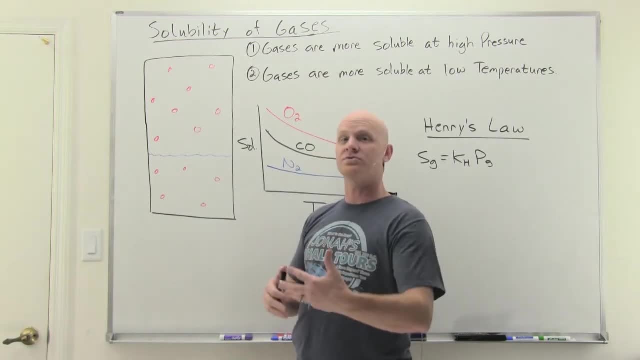 again, what do fish breathe? Fish breathe oxygen, and they breathe oxygen that's actually dissolved in water, And so gases totally can be dissolved in a liquid. So, and it turns out, their solubility depends on a couple of things, and that's both temperature and pressure, And so gases are going to be more. 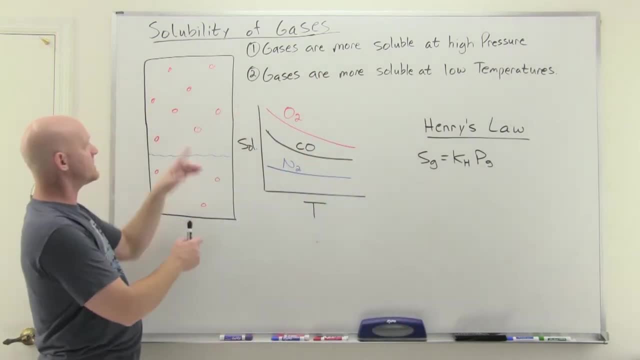 soluble at high pressure. So if we start with that one to kind of look at a gas here, we've got this gas above, say, water, and some of that gas actually dissolves in the liquid And it turns out you establish an equilibrium here, So between the two, and so the more of this gas you put up here, 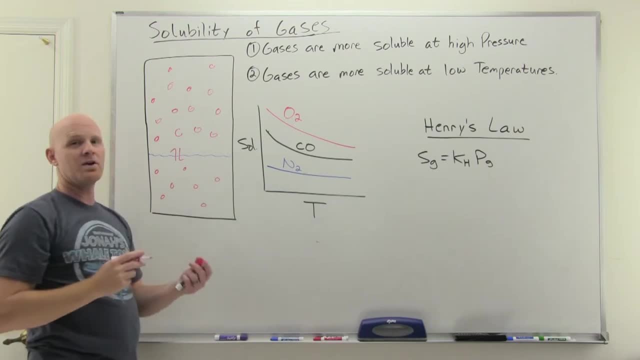 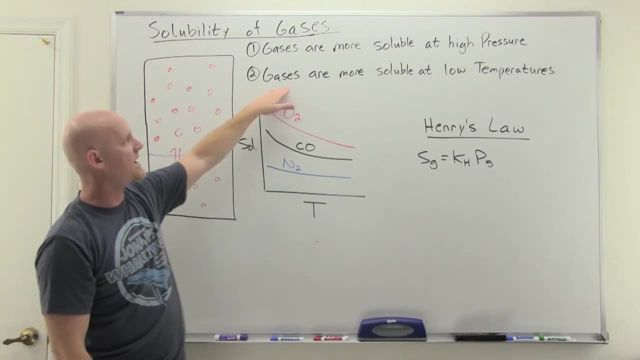 it shifts this equilibrium to get a little more down here as well, And so that's why you get a greater solubility if you have a greater pressure of the gas above it, So, and it turns out gases are more soluble at low temperatures. We can kind of see that on this. 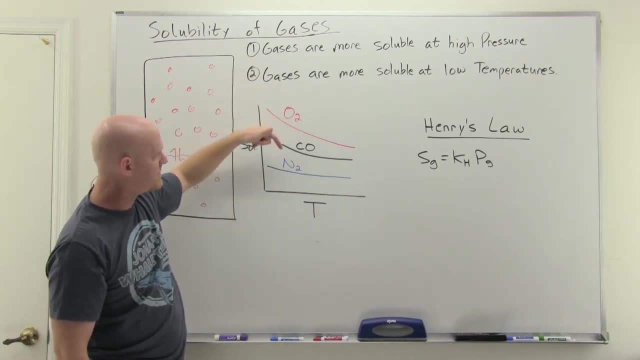 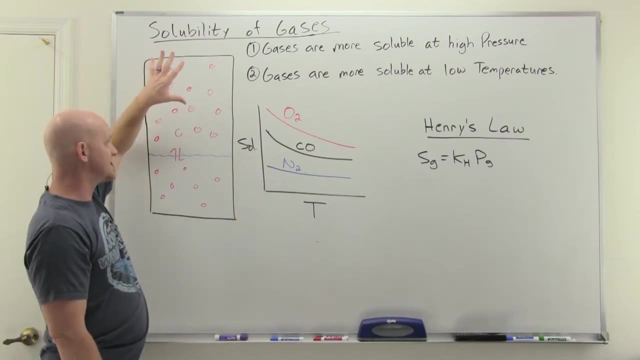 graph here that as temperature goes up, the solubility of O2, carbon monoxide and nitrogen all decrease at higher temperatures, And kind of think of it this way. So if you look at kind of these gaseous atoms or molecules in the gaseous state versus when they're aqueous- here 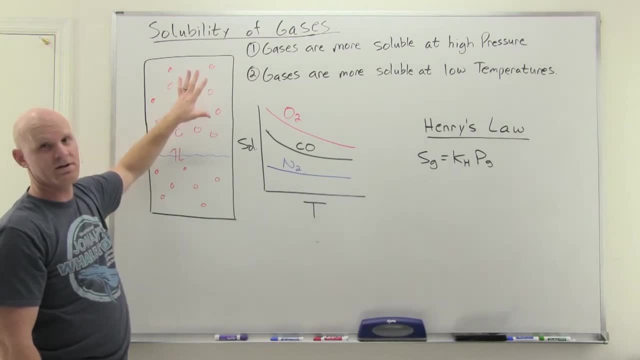 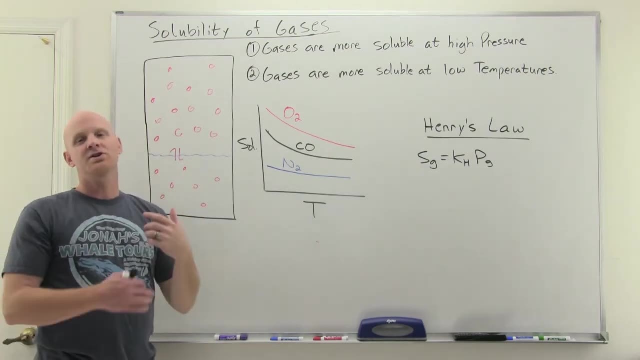 so they're going to have more kinetic energy at higher temperatures. I'm sorry. they're going to have more kinetic energy when they're in the gas phase, Then when they're going to be in the aqueous phase And as you increase the temperature. 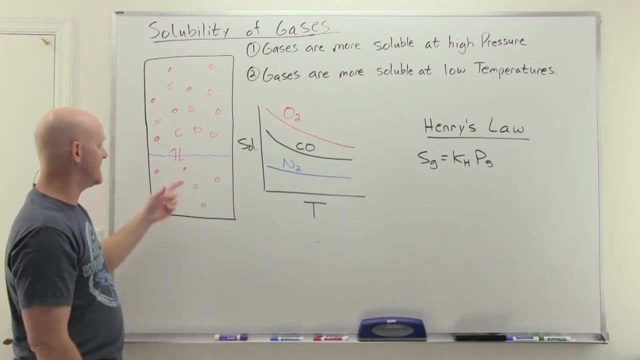 you start giving the molecules in general more kinetic energy, And so some of these ones that are dissolved down here are going to break free of the intermolecular forces holding them in there and end up preferring to be in the gaseous phase instead, And so at high temperatures you get more. 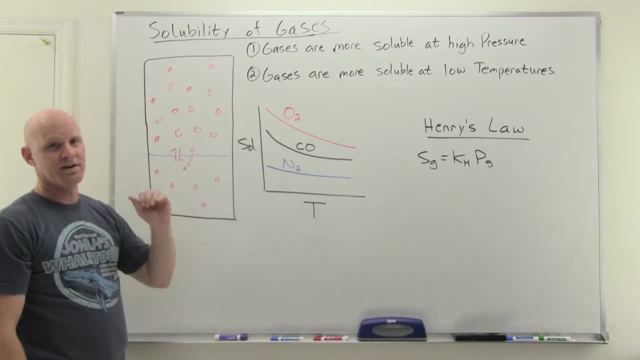 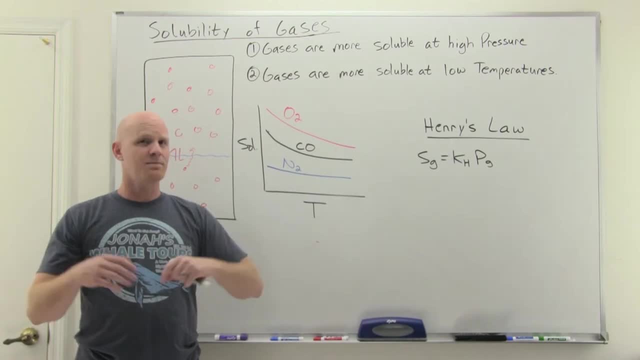 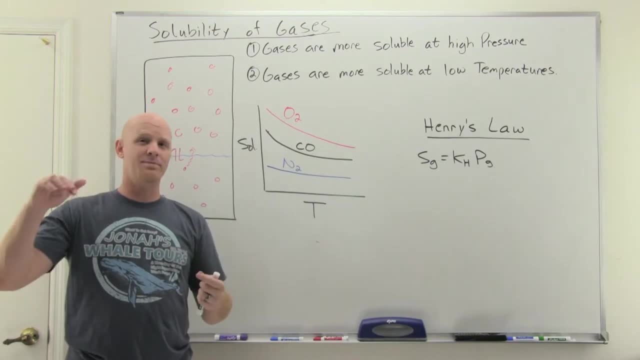 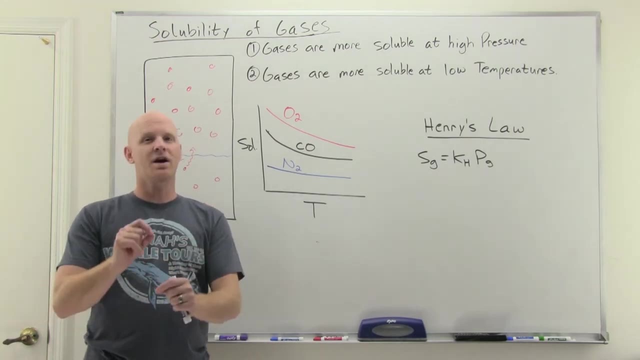 30 seconds or a minute. It's probably going to take five to 10 minutes to get that boiling and stuff like that, Even with your stove on high. what you will notice, though, is that, long before it ever actually boils, you'll see little bubbles coming off the bottom of your pan, And that's not like 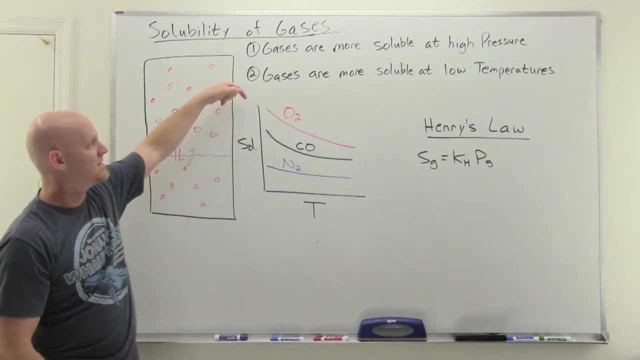 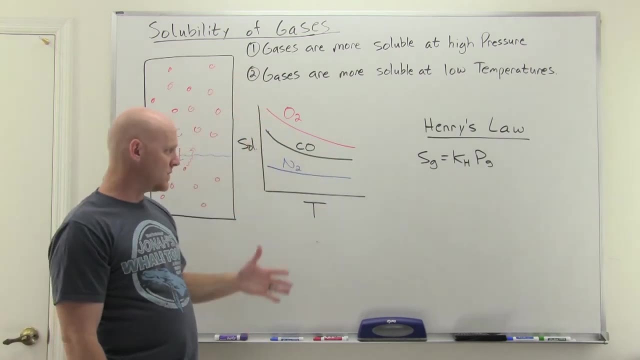 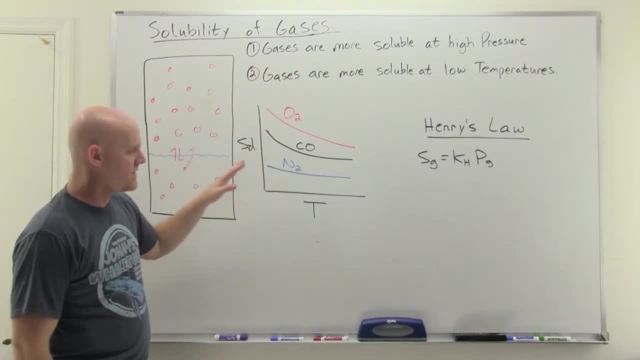 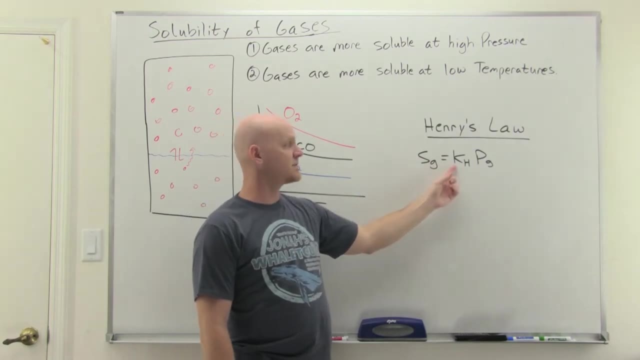 are more soluble at high pressures but low temperatures. So there's also something that we can quantify it with. We call it Henry's law, And so the solubility of a gas in a liquid so is equal to some form of Henry's law. constant times the partial pressure of that gas. above that, 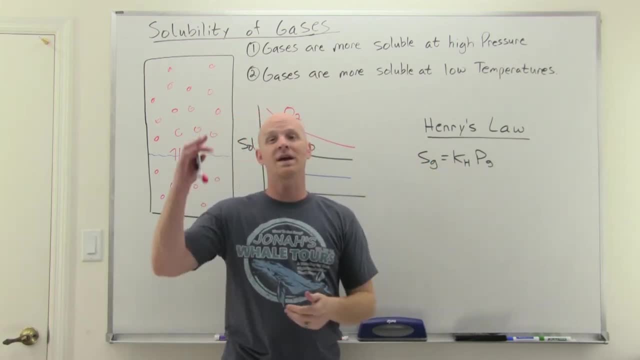 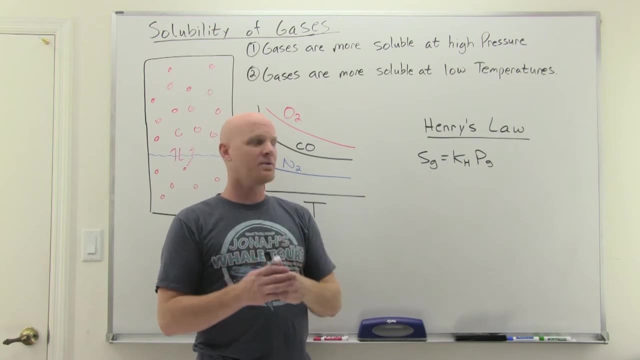 solution. So it turns out these Henry's law constants are specific for a solute solvent pair and they're also temperature dependent, as we see that solubility is totally temperature dependent as well. So but for example, if you looked at the Henry's law constant for oxygen gas, 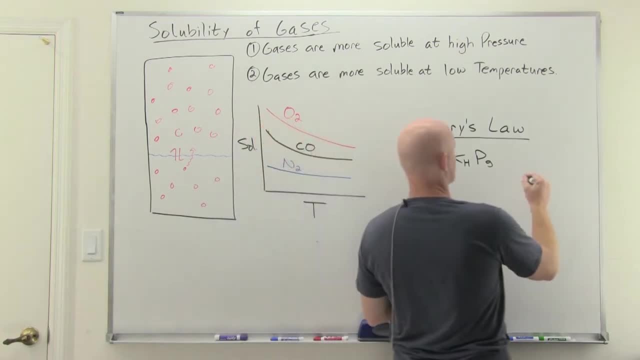 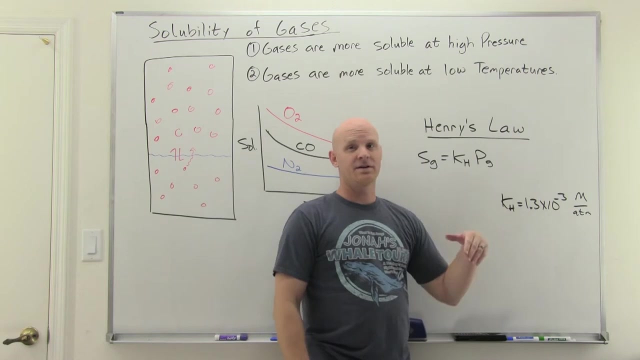 O2 gas at 25 degrees Celsius room temp, you'd find it is 1.3 times 10 to the negative three, And the units on this are molarity per atmosphere. So what this essentially means is that for every one atmosphere of gas- of that, in this case, oxygen- that you have, 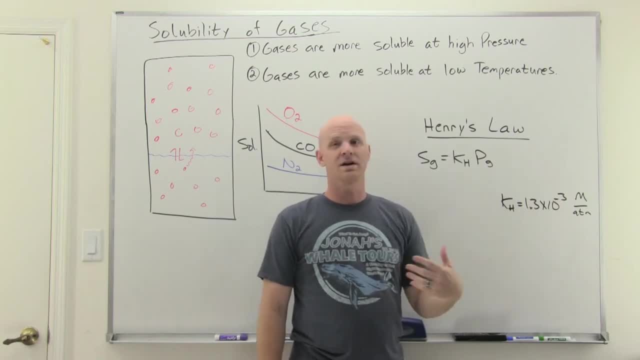 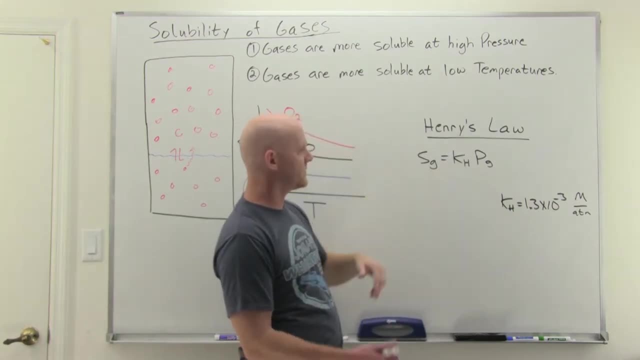 above the liquid, you'll get this molarity to dissolve. And so if you had two atmospheres pressure of O2 above the solution, you'd get double this number of molarity there. so on and so forth. And that's what this equation ultimately means. Now, sometimes they don't actually express it as 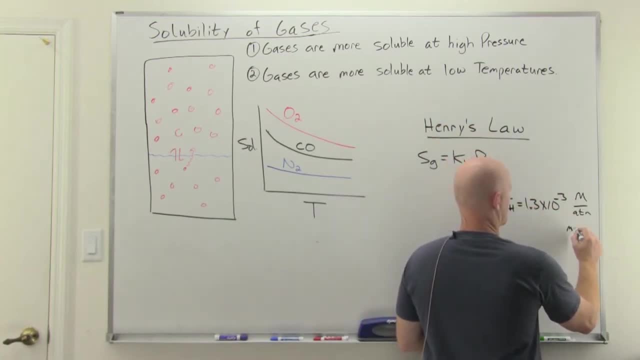 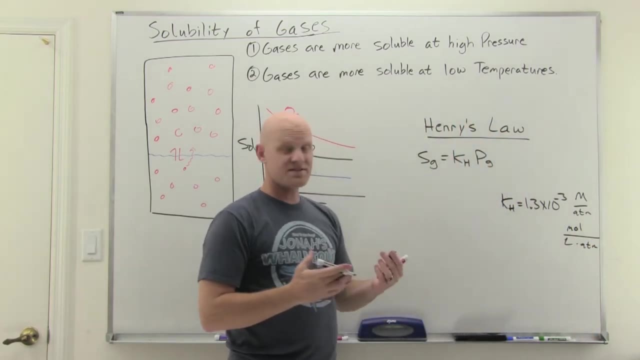 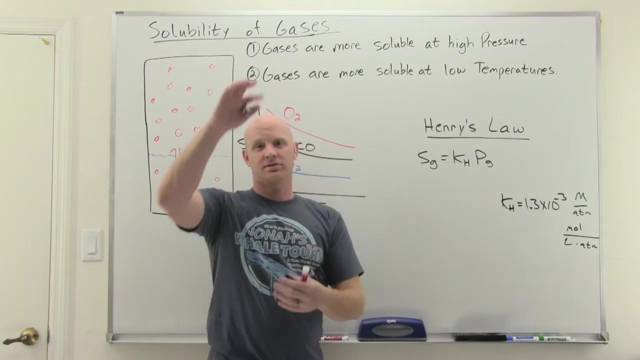 molarity per atmosphere. They break molarity up and you get moles per liter per atmospheres. but you should realize that is exactly the same thing. So if I said, Hey, what is the solubility of oxygen gas in water at room temperature, So at sea level? so you'd say: 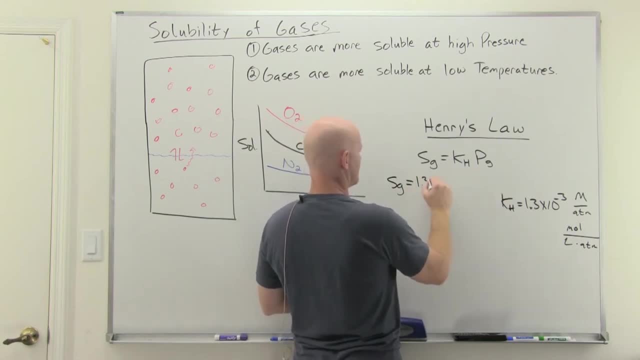 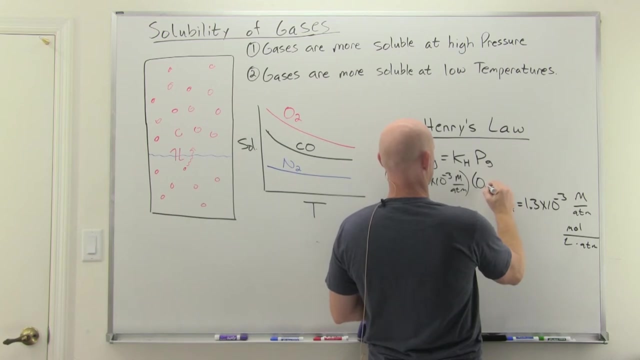 okay, solubility of the gas equals that Henry's law constant 1.3 times 10 to the negative three Molarity per atmosphere. So when at sea level we've got a total pressure of one atmosphere but the partial pressure of oxygen there's just 0.21 atmospheres approximately. 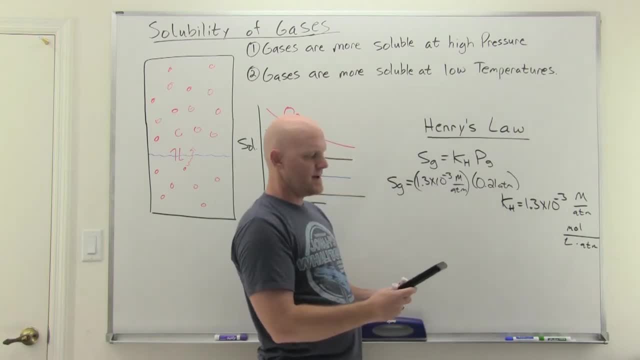 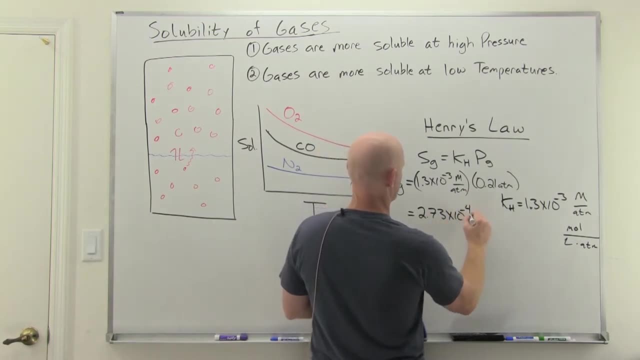 So we can multiply that through- And fortunately I've already done this on my calculator- And this was given us a molarity in the water of 2.73 times 10 to the negative four molar. This would be the solubility of O2 gas in water. This would be the solubility of O2 gas in water. 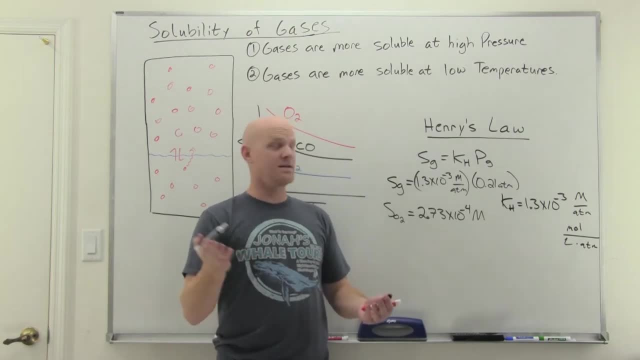 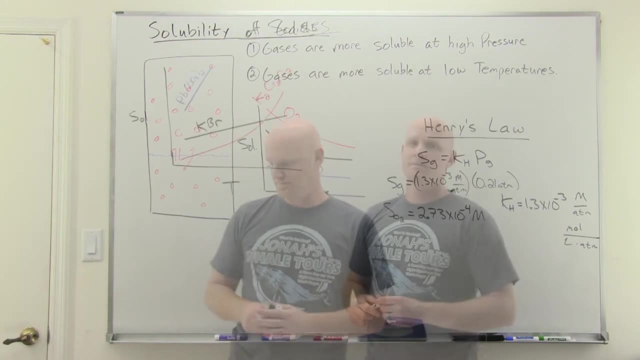 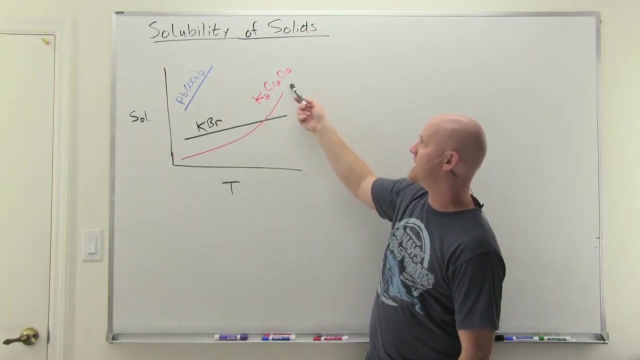 So that's the solubility of gases. Let's take a look at the solubility of solids. All right, So we'll take a look at the solubility of three ionic solids here, So lead nitrate, potassium bromide and potassium dichromate, And you can see that in general though. 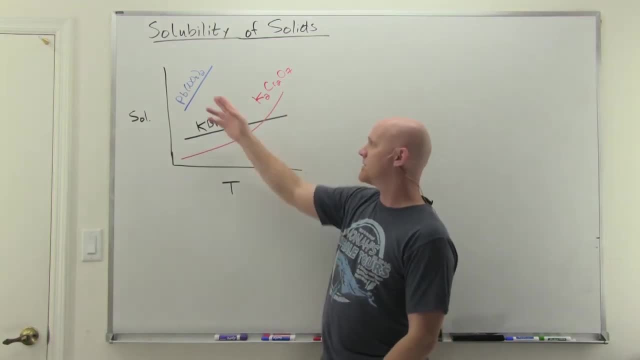 all of their solubility increase at higher temperatures. Some look more linear than others, Some look a little more logarithmic, but they all increase at higher temperatures. Now I didn't pick cherry, pick these or anything like that, but for the vast majority of ionic solids, 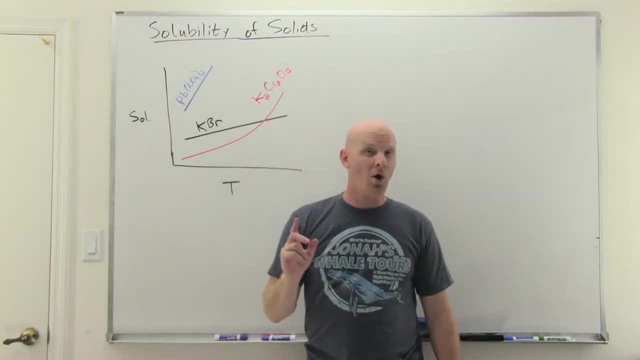 their solubility increase at higher temperatures. There are a couple of exceptions out there, but as a general rule we expect most ionic solids to have their solubility increase at higher temperatures. Cool, We're not going to quantify this in any way, just qualitatively we want to. 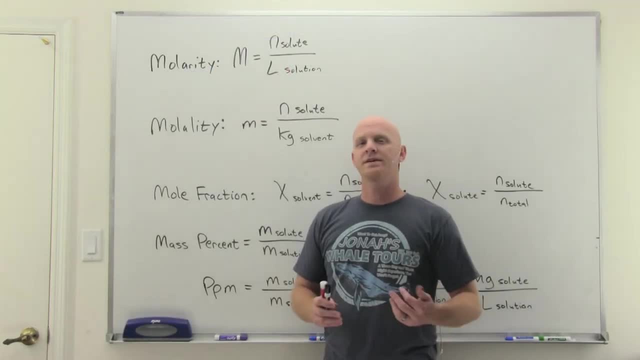 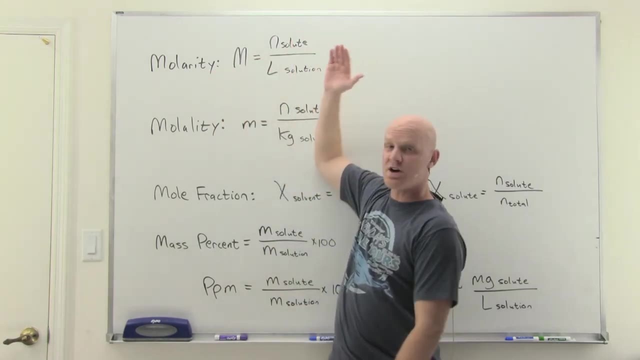 take this concept home. All right, We want to take a quick look at the various ways we measure concentration in chemistry and malaria. you've pretty much already learned So, and it's the most we measured in chemistry, but in this chapter on solutions, so some of the others are gonna be very 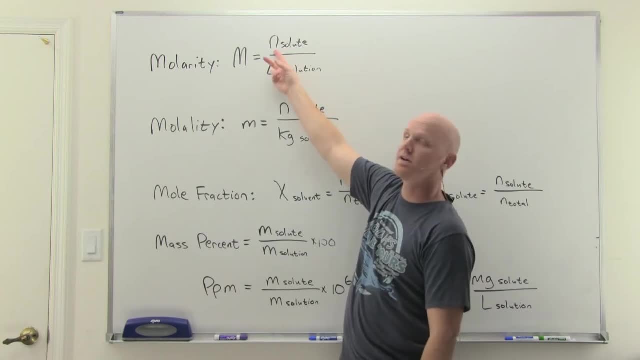 important. So but, reminder, molarity is moles of solute, So, and I'm using here to represent moles over liters of solution, So the entire volume of the solution in liters. So what's new probably to you in this chapter is molality, And so molality, not capital M, like molarity is lowercase M for. 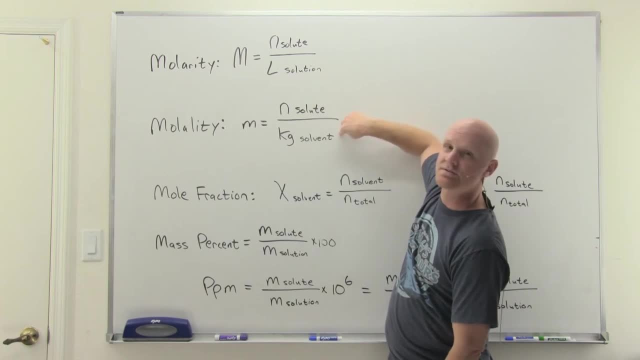 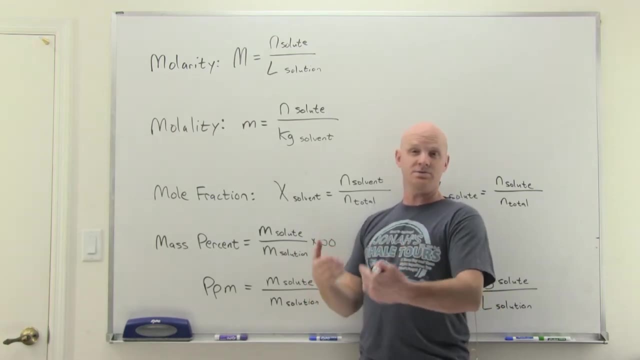 the symbol So, and in this case it's moles of solute instead of over liters of solution, it's just over the number of kilograms of solvent. Now it turns out for dilute aqueous solutions. So solutions in water where you don't have a lot of solute. molarity and molality often are pretty. 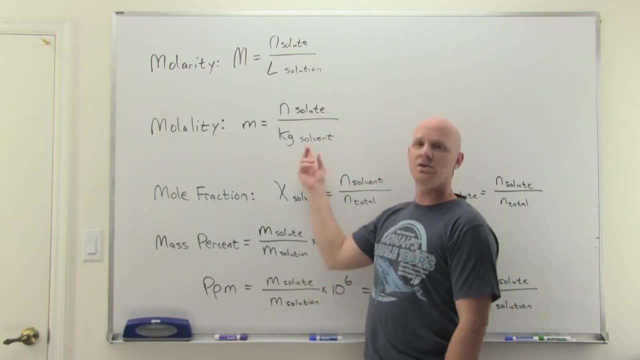 close to exactly the same number, And the reason they are is that one kilogram of water, So it happens to be one liter of water as well, And so as long as there's not a lot of solute, so pretty much the liters of water would be pretty close to the leaders of the entire solution, And so the 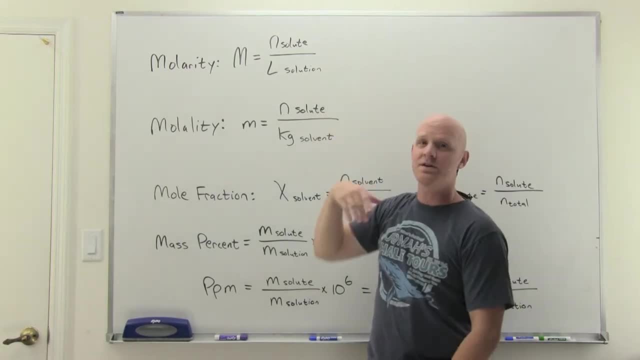 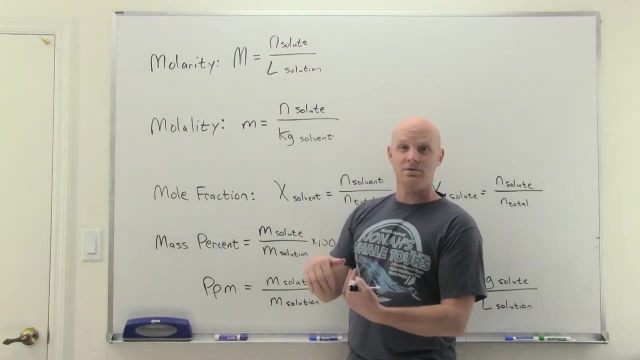 leaders of solution and the kilograms of solvent would be pretty darn close to the same thing. Now, as you get more and more solute, though, these two numbers are going to deviate, because as you add more and more solute, your solution's going to get bigger, but your kilograms of solvent isn't. 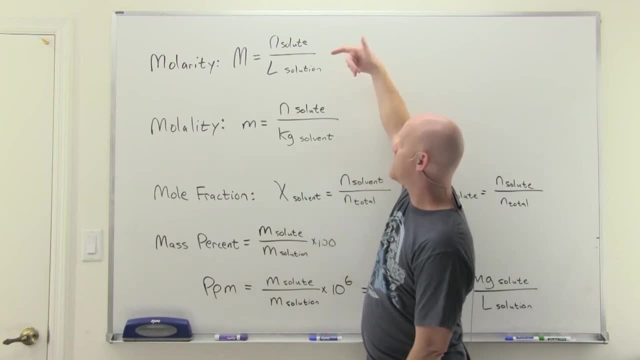 going to change at all, And so, as you add more and more solute. so, because of the dominator up here getting bigger and bigger and bigger, your molarity is going to end up lower than your molality for more concentrated solutions. Cool, This molality is important, though We're going. 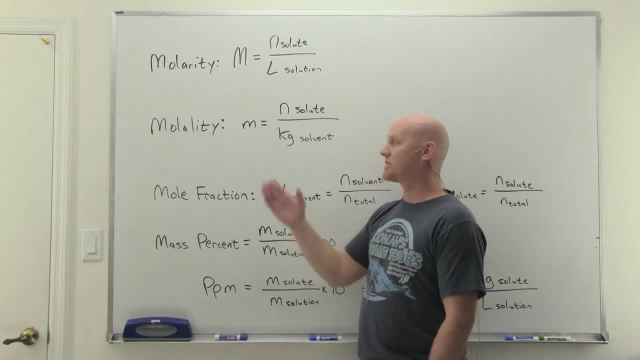 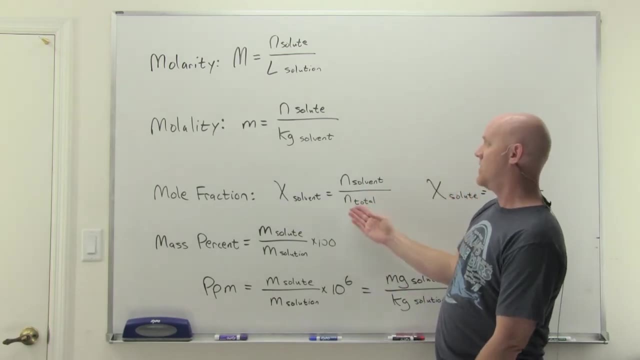 to use this in some of our colligative properties that we'll study in a little bit, And so that's why it's being introduced right now. So mole fraction is very similar, And you could talk about the mole fraction of the solvent, which would just be the moles of solvent. 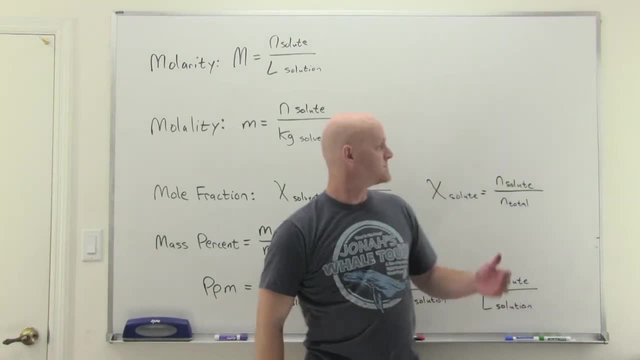 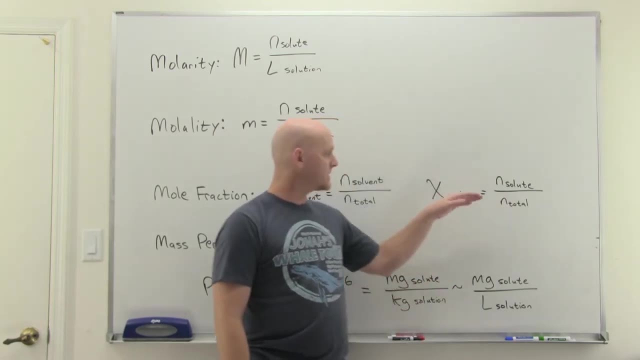 combined, ie the total moles. Or you could look at the mole fraction for the solute and it would be moles of solute over again, moles of solute and solvent combined, the total So, and you could look at either one of these and we'll see that we're going to find the mole. 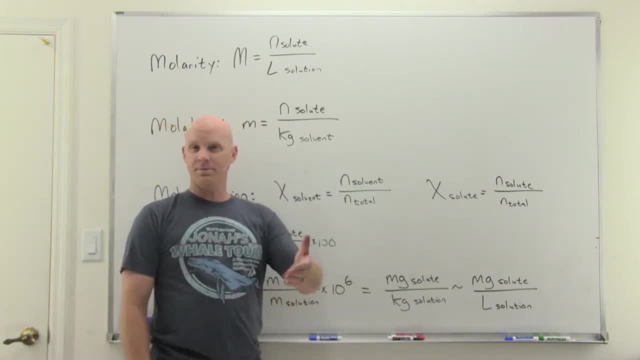 fraction of the solvent when it comes to Raoult's law, with vapor pressure depression, one of our colligative properties, and hence the relevance here. But this isn't the first time you've seen mole fractions. You saw them with Dalton's law of partial pressures as well, in dealing with gases. 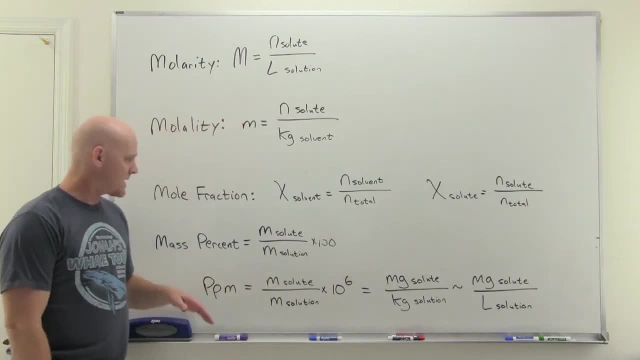 Now we're bringing it up with solutions here. All right, finally we've got mass percents and you guys are probably pretty well familiar with how you find a percentage. You take the part over the total times a hundred and that's a percent. 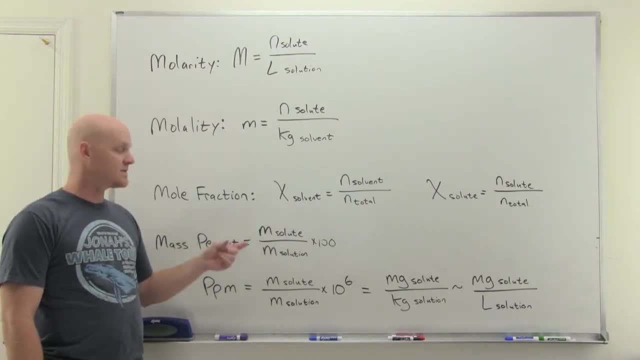 So in this case, if I want the mass percent of solute, I just take the mass of the solute divided by the total mass of the solution, solute and solvents combined. so in times a hundred, Cool, And that's a mass percent. So one thing you might not. 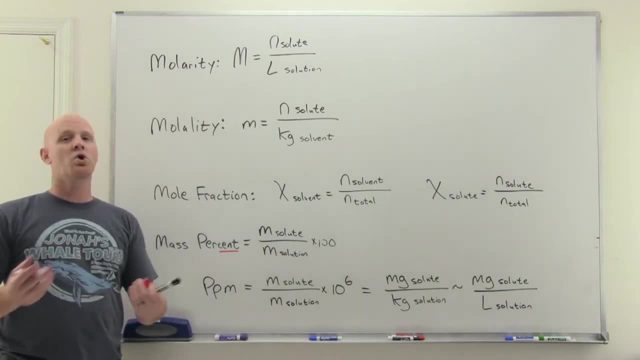 recognize, though, is that a percent is always a per 100. And so, to find a percent, you always end up multiplying by a hundred at the end. Now we're going to talk about parts per million. Sometimes, at even more dilute solutions, we talk about parts per billion, and it is just. 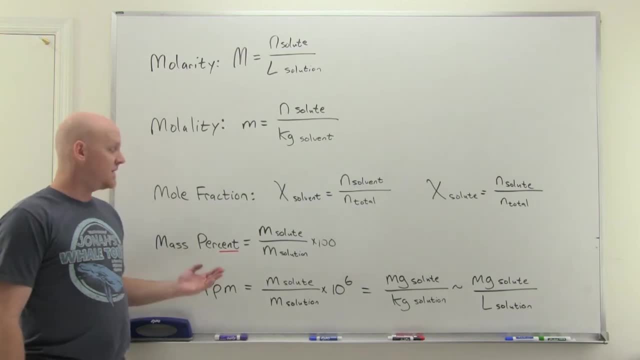 like a percent, except instead of multiplying by a hundred at the end with parts per million you multiply by a million at the end. If you were doing parts per billion, it would be multiplying by a billion at the end of the calculation here, But it's still just mass of solute part over. 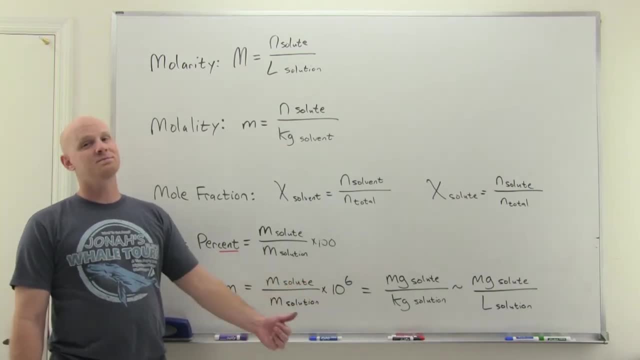 the mass of the whole solution total times instead of a hundred times a million for parts per million. here Jacob's Law of Solute Parts per Million and Solvents combined part per million. Now, often this works out instead of expressing it like this, which is what it is and makes: 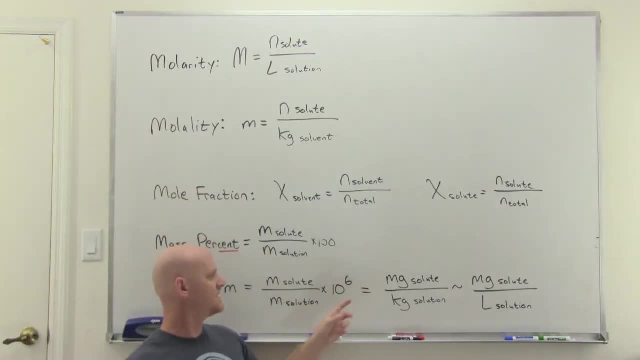 sense to me personally, So we'll often express it like this instead- and factor in this 10 to the 6th right from the get-go, and we'll take the milligrams of the solute over the kilograms of solution, And the idea is that milligrams and kilograms are different by a factor of 10 to the 6th. 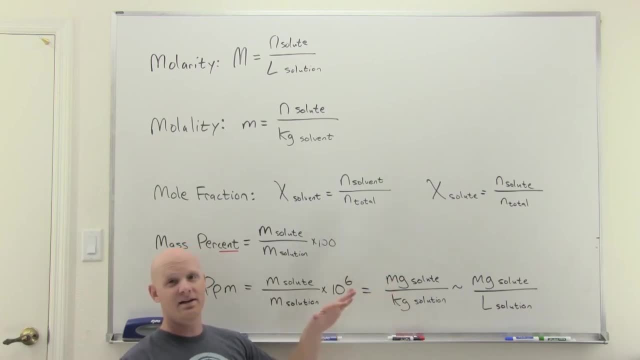 and it already accounts for this part of it, which is why it's not needed. And so, if you already just know your kilograms of solution, milligrams of solute, rather than finding their masses in the same units and then multiplying by 10 to the 6th, you 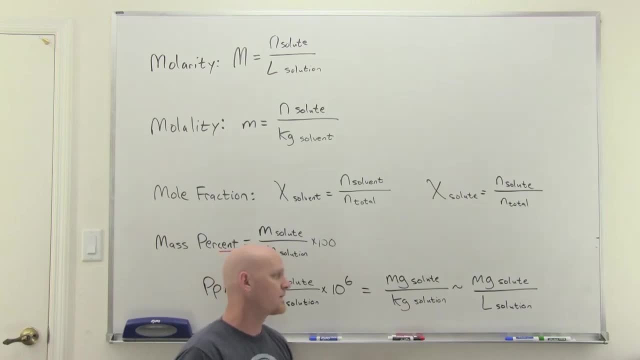 can just go milligrams over kilograms and be done right from the get-go. Now, if you're dealing with aqueous solutions, if you recall, we also said that water. again, one liter of water weighs one kilogram. And as long as we're talking about fairly dilute aqueous solutions- oftentimes this 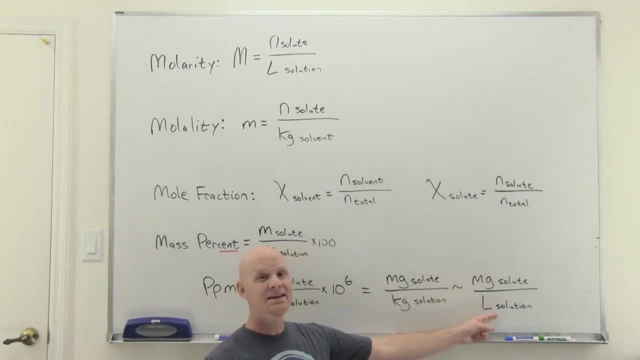 gets reduced down to milligrams of solute over liters of solution as well. So you'll see this used quite ubiquitously, although for more concentrated solutions maybe we shouldn't be using it So, but it's almost exactly the same thing as what we had right here again for dilute. 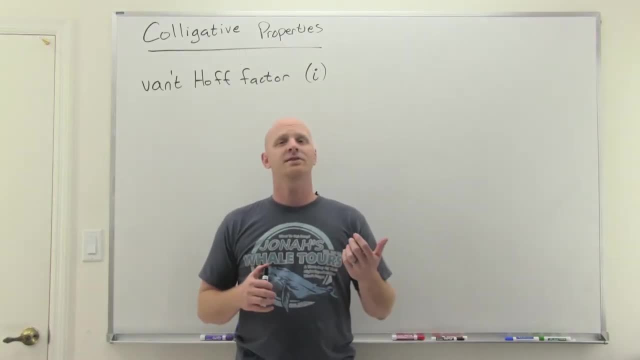 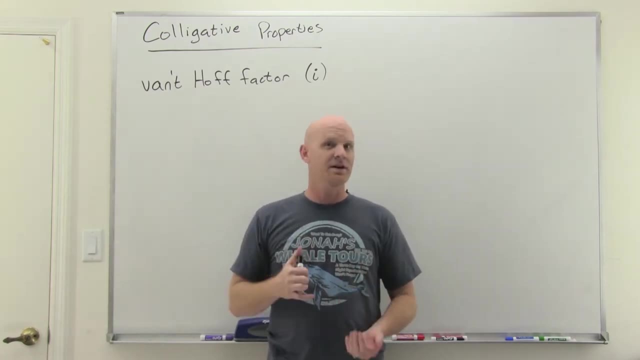 aqueous. So now we're going to have a fairly comprehensive discussion of colligative properties. Now, a colligative property is a property of a solution that, as you add solute, it changes more and more. The more solute you add, the more it changes. 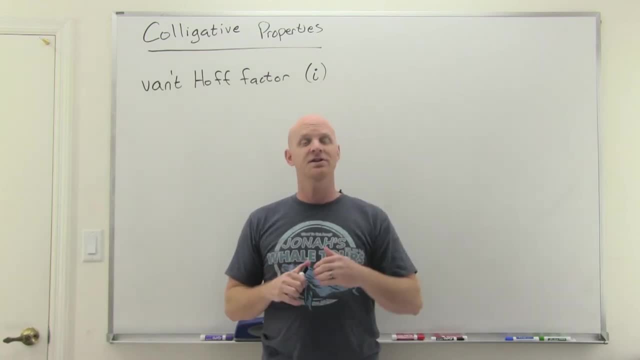 So, and these include things like freezing point depression, boiling point elevation, vapor pressure depression, which is governed by Rawlitz law, and finally, osmotic pressure, which we'll deal with when we get there. So, for example, let's say you had some water. 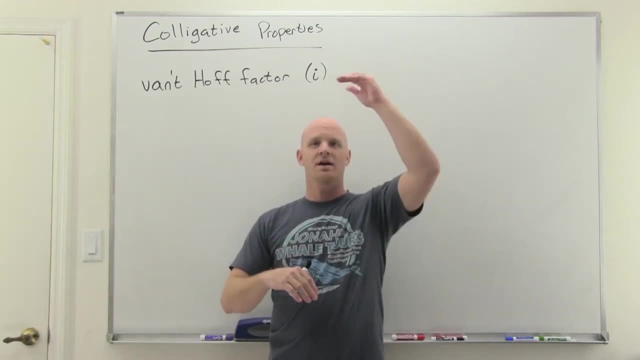 So normally pure water has a freezing point of zero degrees Celsius And a boiling point of a hundred degrees Celsius at one atmosphere. Now, let's say, instead of pure water, now you start either pouring in some sugar or pouring in some salt, just pouring in some solute that's going to dissolve. 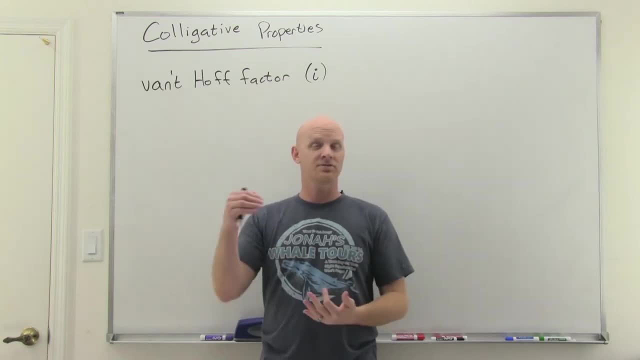 And largely the identity of the solute is not going to be important as long as it dissolves in the water, And what you'll find out is that after you pour some solute in the freezing, point's no longer going to be zero. 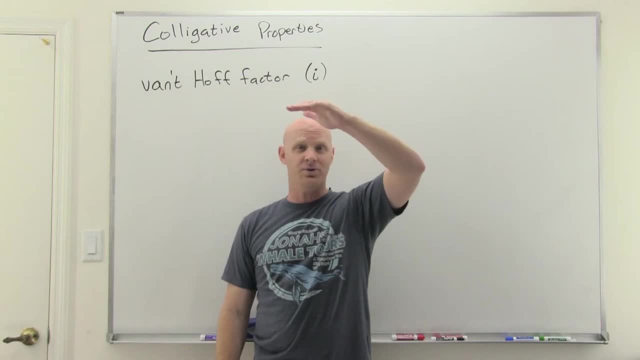 It's going to be lower than zero degrees Celsius, and the boiling point's no longer going to be a hundred degrees Celsius. It's going to be higher than a hundred degrees Celsius. And what's interesting is, the identity of the solute is not that important. 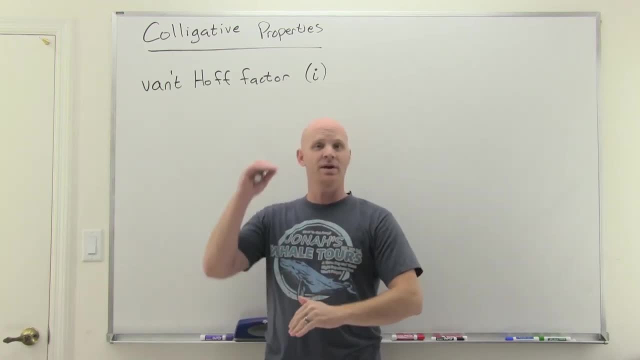 So any solute is going to cause the lowering of that freezing point and the raising of that boiling point. So kind of interesting. If we look, there is one characteristic about the solute that is important. It's what we call the Van't Hoff factor. 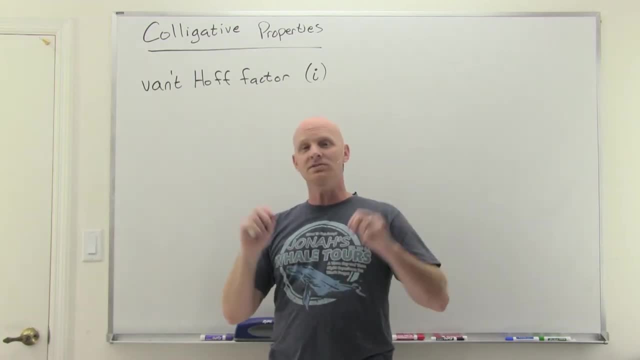 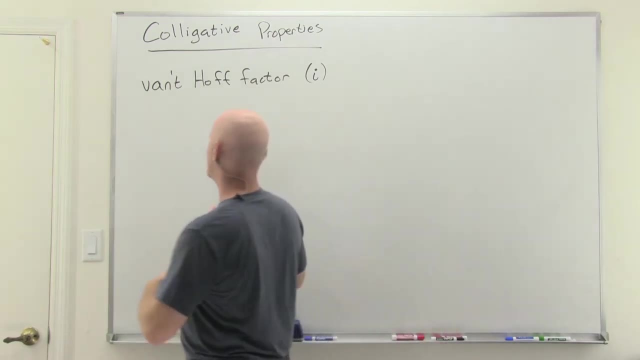 And it turns out the Van't Hoff factor just gives us a description of how many pieces a particular solute dissociates into, In this case an electrolyte, how many ions it dissociates into. So if we start with something like, say, methanol or maybe glucose, 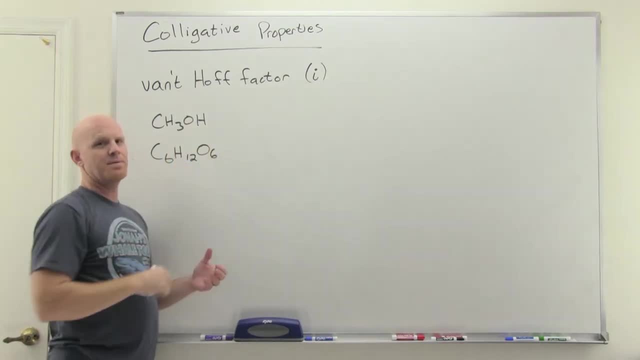 So these are molecular compounds and they're molecular compounds that are not acidic or basic. And back in chapter four you learned that they are non-electrolytes, And for a non-electrolyte it doesn't dissociate into ions at all. 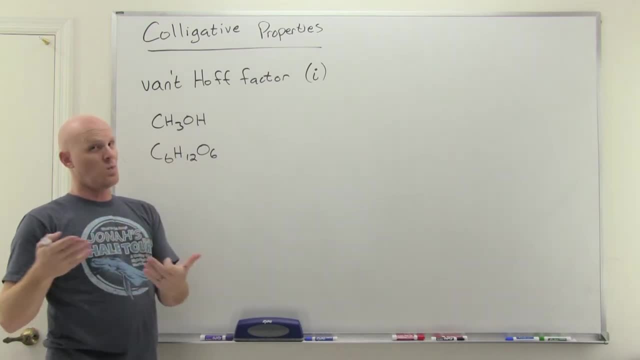 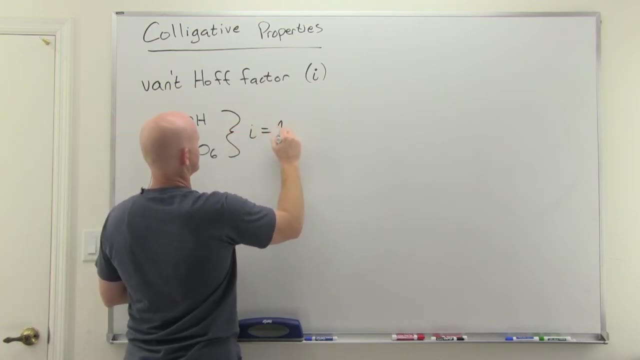 And so for every molecule of either one of these you get, you get one dissolved piece in your solution. And so as a result, for non-electrolytes, your Van't Hoff factor is simply one: Every molecule provides one dissolved particle. 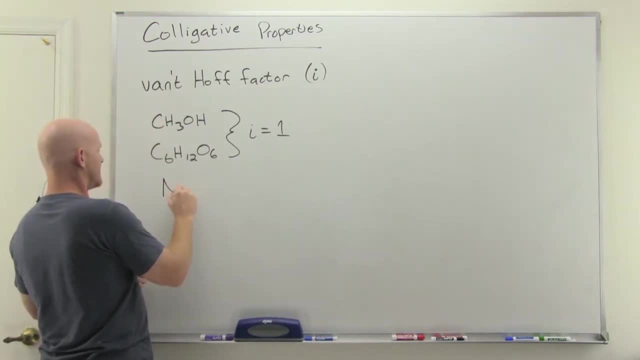 That's it Okay. So move on to some electrolytes here, And we'll go on to strong electrolytes that dissociate into ions completely, so something like NaCl. NaCl dissociates to give one single sodium ion and one single chloride ion, but two total. ions, And therefore the Van't Hoff factor is going to be two. Let's make this a little more complicated. Let's put something with polyatomic ions in there. So aluminum nitrate is another strong electrolyte. dissociates completely into ions. 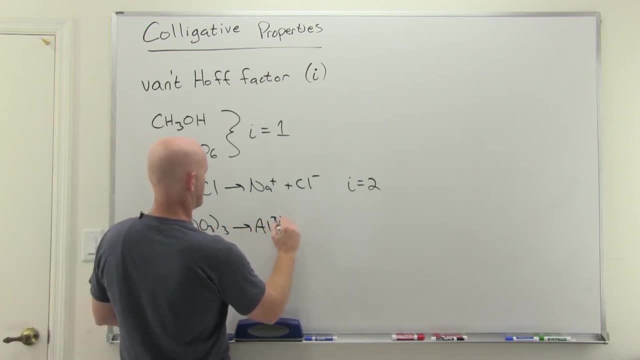 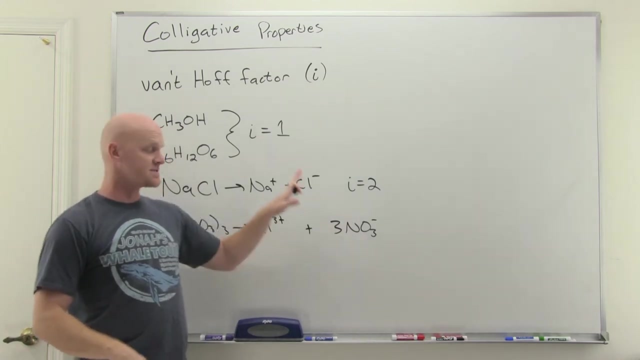 The cation is aluminum and you get one of those. But nitrate is the anion and you get three of those. But notice, the polyatomic ions themselves don't split apart in atoms or anything. That's one of the mistakes students make, is they try to start splitting apart the polyatomics. 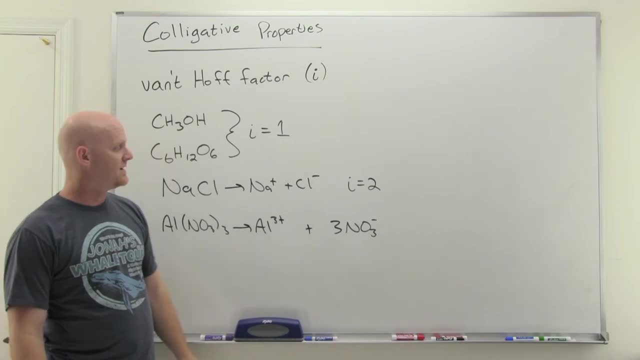 But it's just cations and anions separate but don't break up any polyatomics further than that. But we got one cation, four anion, I'm sorry, one cation, three anions, a total of four. 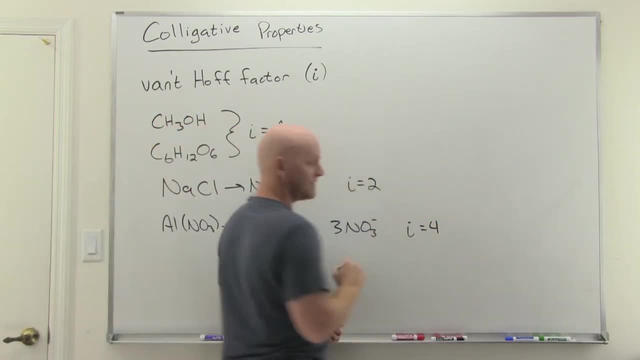 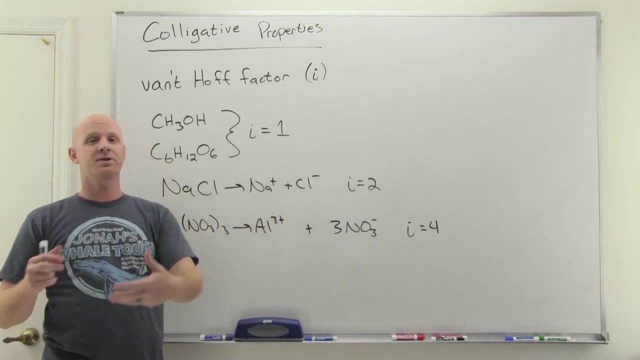 ions. Okay, So Van't Hoff factor is four. Cool, And so just by visual inspection, as long as you know something's a strong electrolyte, you can kind of predict how many ions it's going to split apart into, and therefore predict. 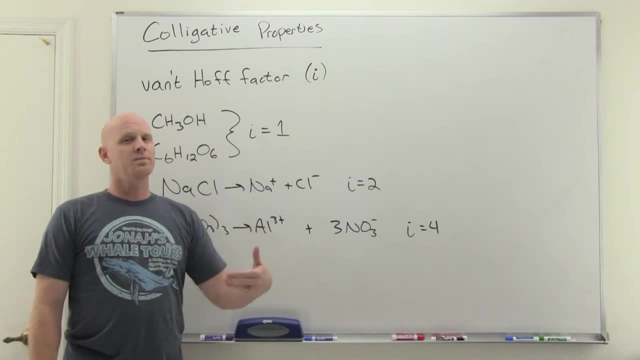 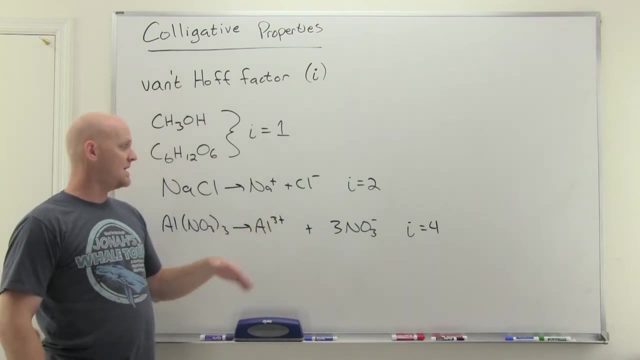 its Van't Hoff factor, And the idea is it's not just the total molality we'll find out of the solute, but it's going to be the total concentration of all dissolved species, And so if it splits apart into multiple pieces, we want to factor that in. 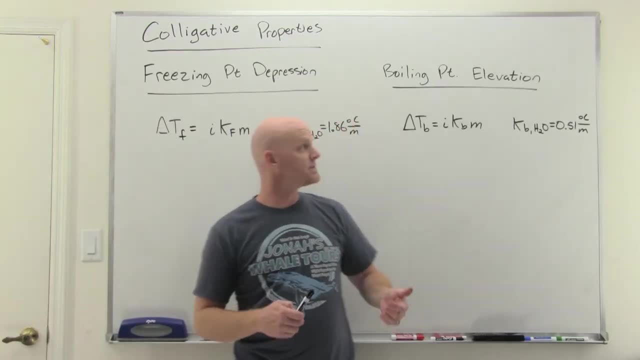 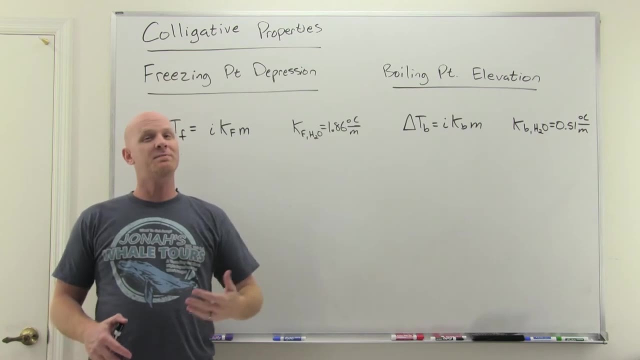 All right, now we'll take a specific look at freezing point depression and boiling point elevation. So freezing points do indeed go down, boiling points go up, and we want to talk a little bit about why, and then we'll get into the math of it here. 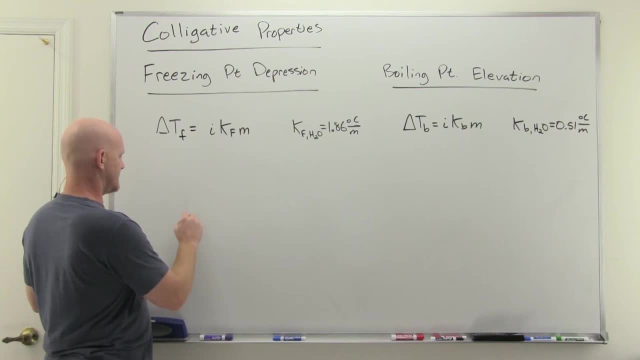 So let's say you've got a crystalline substance here and it freezes into a nice pretty crystal structure here, Cool. So what happens is the molecules, let's say in the liquid phase, are moving around and stuff like that. 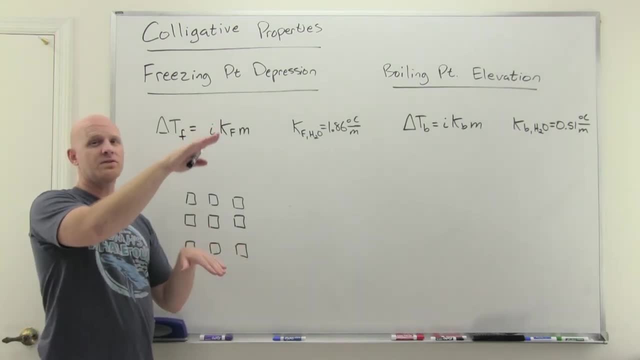 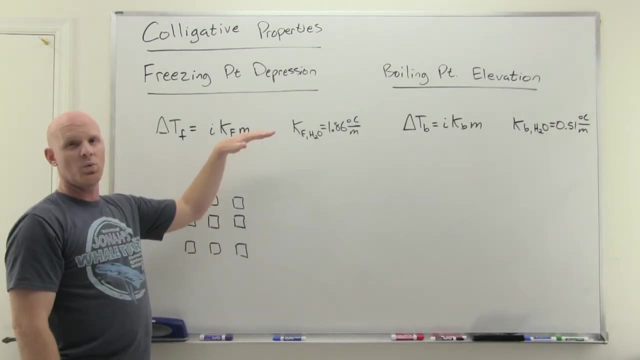 And as you lower the temperature, they slow down. So, and at some point you've slowed down, Okay, So you've slowed it down enough that the intermolecular forces take over and lock it into place. So, but this is only going to happen when they slow down enough. 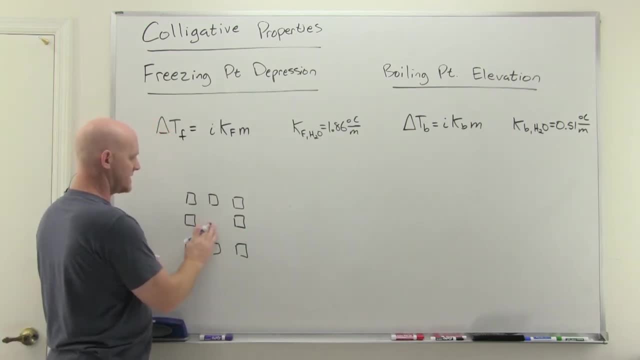 Well, once you stick an impurity in there, of any sort, the impurity, it doesn't matter what it is, as long as it's not the same thing as the solvent. And so in this case, I'm just going to put some random impurity in there and represent. 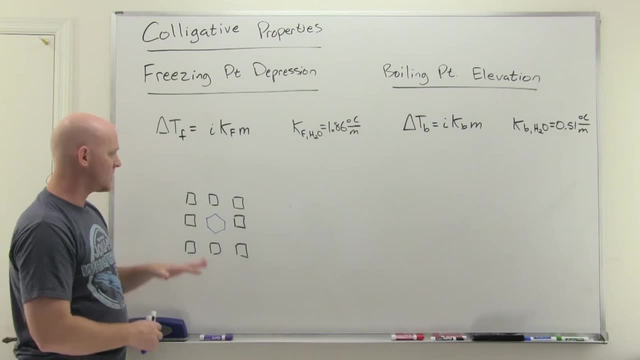 it as being different, with a different color and a different shape. So, and the problem is now, I've put a kink in this crystal. There's something there that doesn't belong in it. It doesn't fit into the crystal structure quite as well. 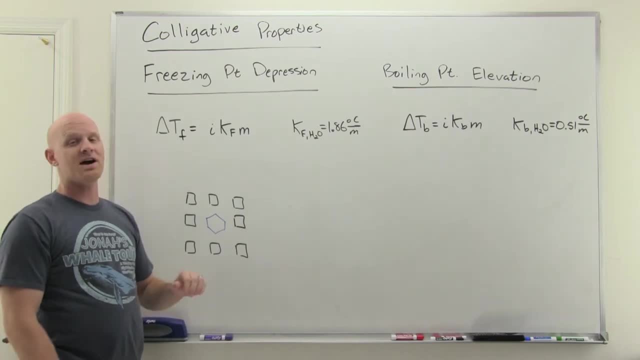 And, as a result, we're going to actually have to cool the solution down even lower than normal to where it will actually freeze into this imperfect crystal. And that's why freezing points get lowered. And you can look at it as freezing points get lowering, but it's also a lowering of 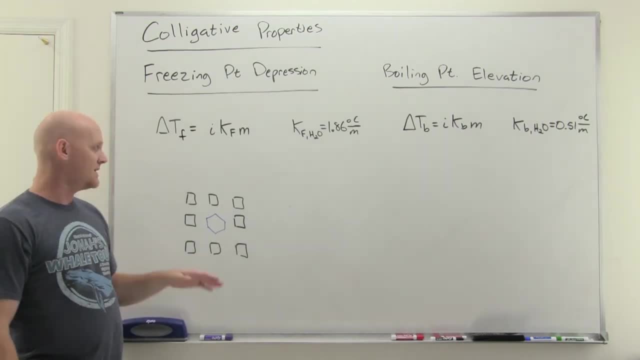 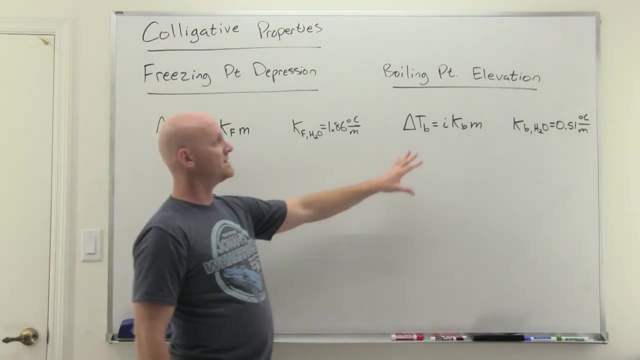 the melting point of the solid, if you want to look at it that way as well. So it works either way. The freezing point and the melting point are one and the same, But this is kind of the crux behind freezing point depression. Now boiling point elevation is going to be a little bit harder to explain. 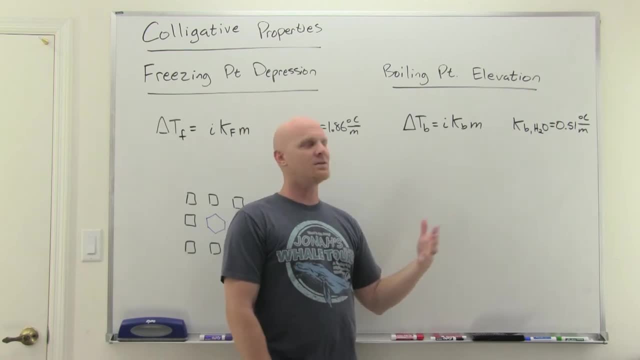 So with boiling point elevation it's not a. you know, a lot of students are taught incorrectly that well, I guess the intermolecular forces are going up when you have the mixture, and that's not true. So what you actually got going on is something a little bit different. 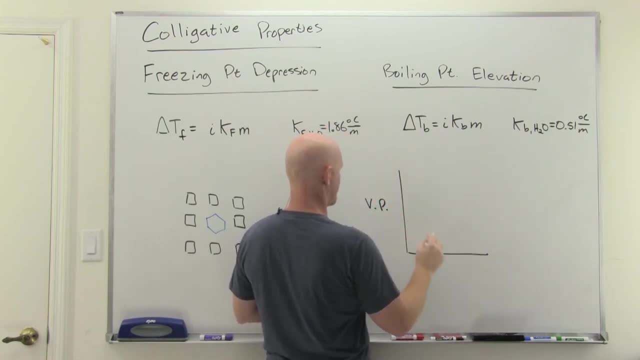 So, if we take a look here, so- and I'm going to plot vapor pressure versus temperature, So and it turns out- this is something you intuitively already know- but vapor pressure goes up as you go to higher temperatures. So, and you know this intuitively- 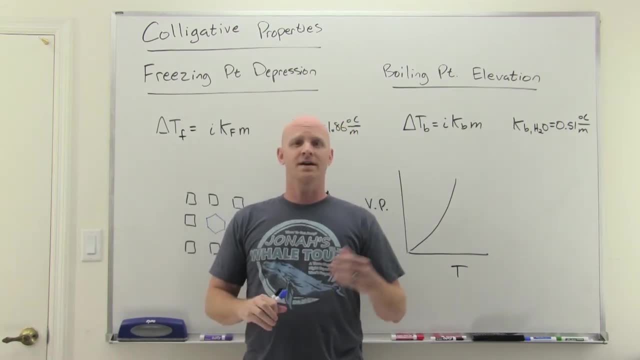 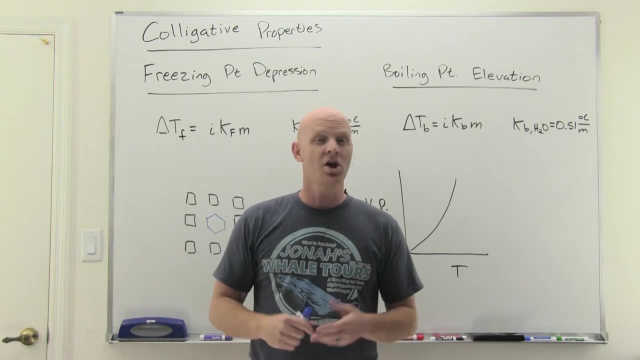 You just don't realize that. you know this. So, but if I gave you the option- and I'm going to put on a plate in front of you, so a turd fresh out of the freezer or one fresh out of the microwave, which would you prefer? So- and I'm reading your mind, you're saying the one out of the freezer because you like them crunchy. I know No, you want the one out of the freezer because it's not going to smell as bad, because as temperature goes up, the vapor coming off that turd is going to be worse. And so the one of the microwave is going to smell a lot worse. So So think about it. It's given off a lot more vapor. for you to smell it, whether it's cold or warm, You have to have poop molecules in your nose, and I'm glad I could ruin your life when you 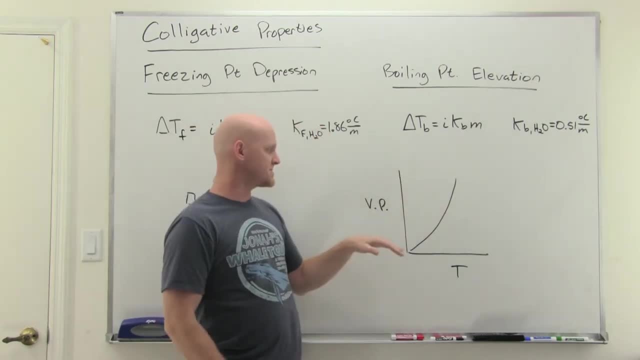 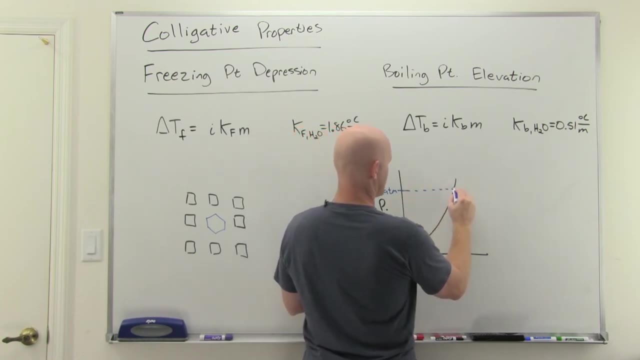 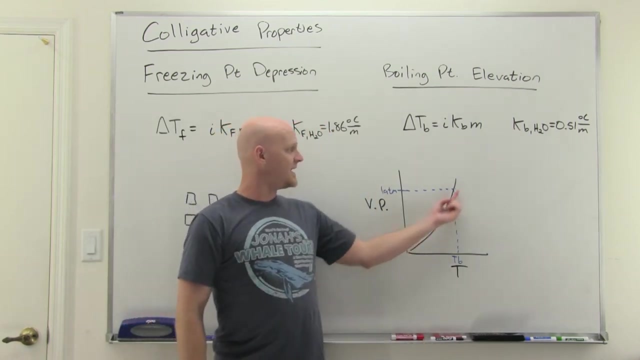 think about that. So, but that's the deal. You get more vapor at higher temperatures and eventually, at some point when you reach one atmosphere, that actually is when a substance boils Cool. So you hit the temperature high enough till you actually hit one atmosphere. 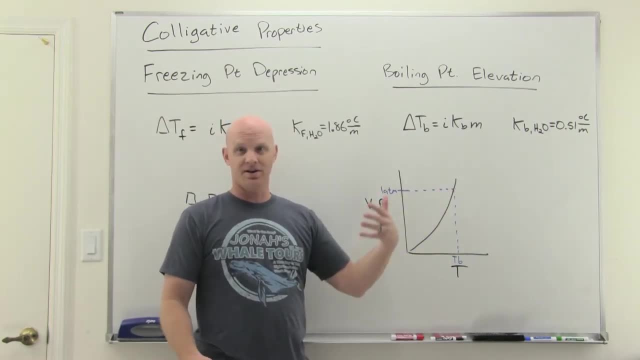 So So you hit the vapor pressure, and that's when you actually reach the boiling temperature And it turns out what's really happening there is once you hit that vapor pressure of one atmosphere. that's when what we call the chemical potential of the liquid and the chemical potential 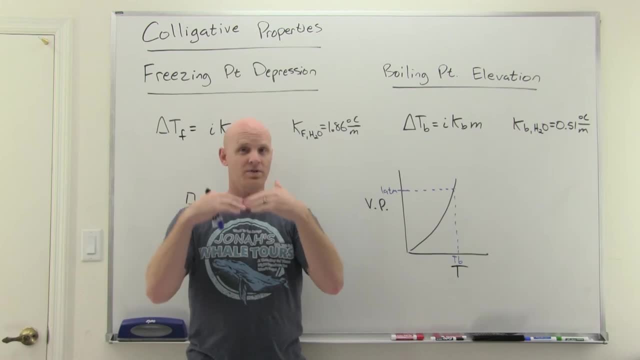 of the gas are equal, So, and it's once they are equal. that's when you actually get it to boil as well. Another way to look at it, So that's more of a physical chemistry way of looking at it. So, but what happens when you add solute? is it changes your curve? 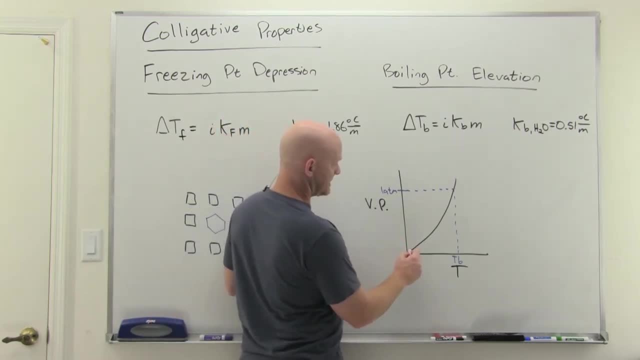 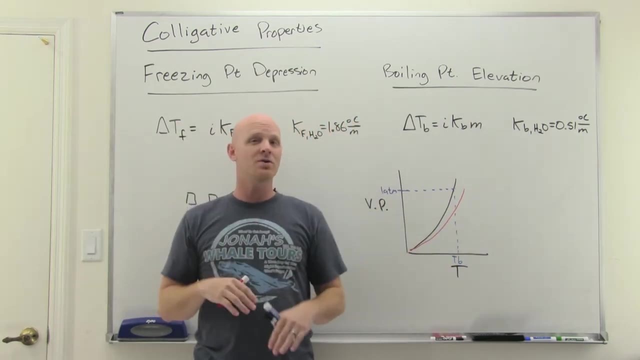 So it actually changes your curve and it shifts it down a little bit. So it turns out, when you dissolve a solute in there, it lowers the chemical potential of the liquid, So so that solid, or whatever solute it is, is going to dissolve and mix with the solvent. in this case water, maybe spontaneously, and that lowers its energy. Spontaneous things always lower the energy and by lowering the energy of the liquid we have to heat it up even hotter than normal, till it actually is has a chemical potential. 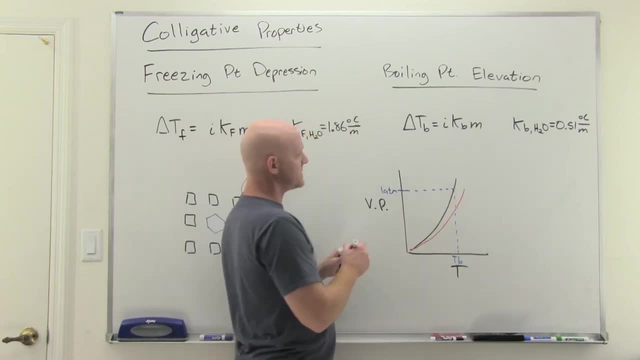 equal with the gas, Or So we don't have it until we actually reach one atmosphere vapor pressure and get this new boiling temperature. So this is not the most satisfying answer in the world of what's going on. It's a little heady. 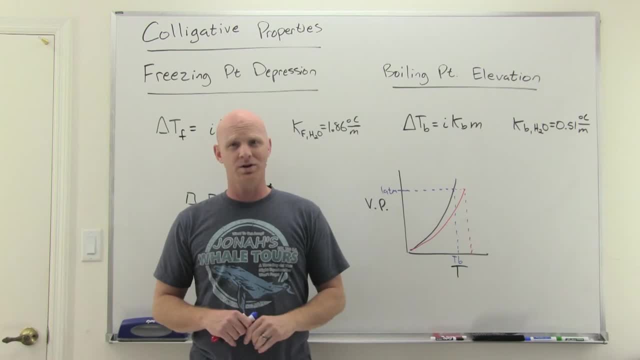 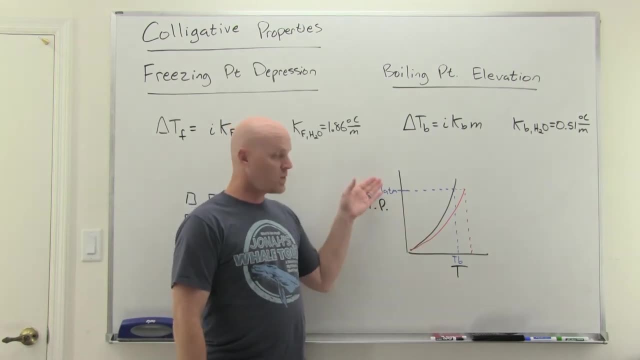 It's just sometimes easier to lie to students and say, oh, the intermolecular forces get bigger when you make the mixture, which is totally wrong. So this is really the real reason. So, but takeaway, here was a good, convenient time for me to teach that you know boiling. 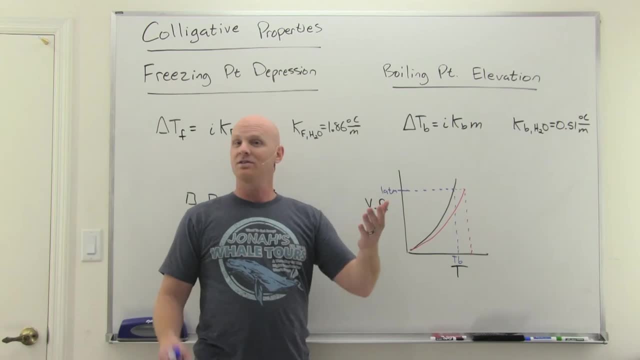 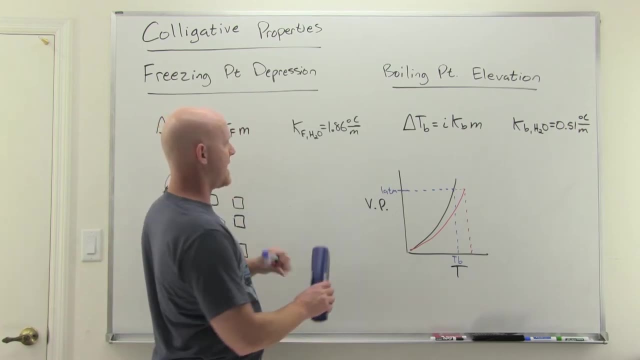 point is really when the vapor pressure reaches the external pressure, So that's kind of a convenient time to teach it and stuff like that. So That's the reason behind boiling point elevation. So let's take a look at a little bit of the math, though, involved with both of these. 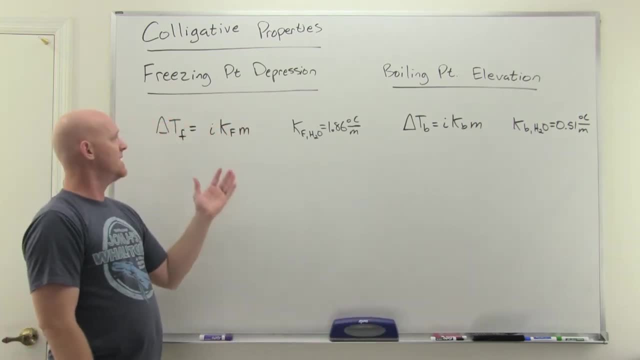 All right. So here's the typical equations you're given. So your change in your freezing point or your change in your boiling point depends on the molality of your solute. If it breaks up into pieces, it'll depend on how many pieces it breaks up into its Van. 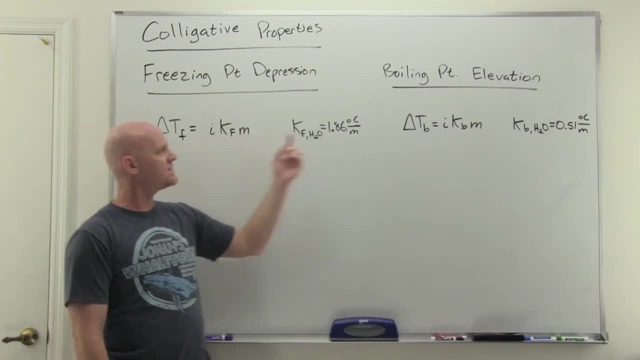 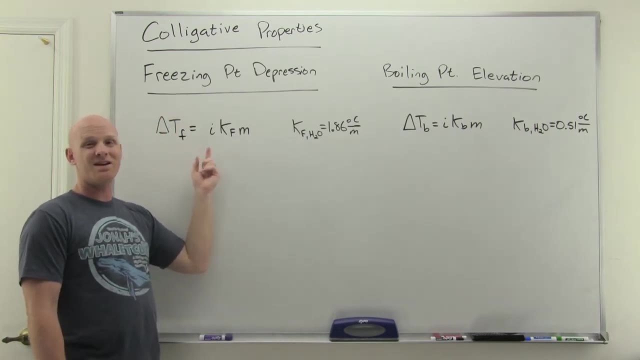 Hoff factor and then a characteristic constant. So either a freezing point constant or a boiling point constant. Now, boiling points go up, And so the change is always going to be positive, But freezing points go down, So the change is always going to be negative. 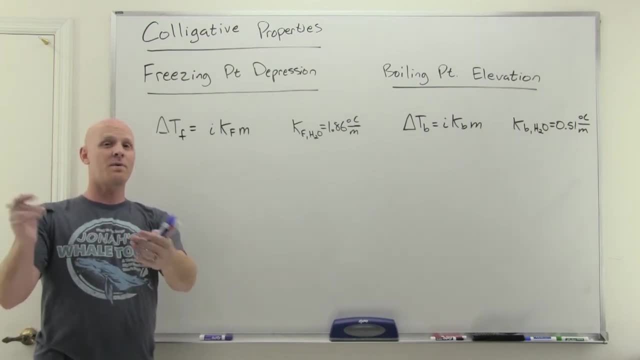 Now, most of the time when they present it it just looks like this And they expect you to remember that it's negative. Personally, I just like putting the negative sign right into the equation. That way, when you calculate the change in the freezing point, it always goes down. 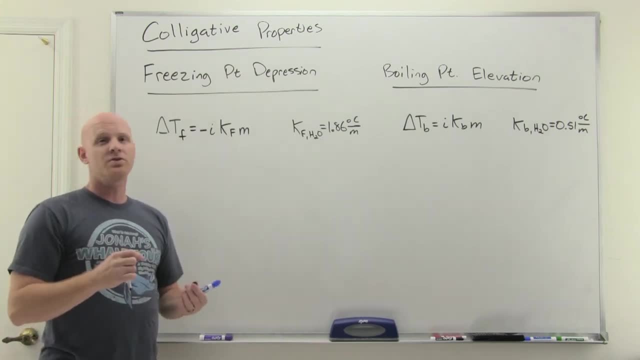 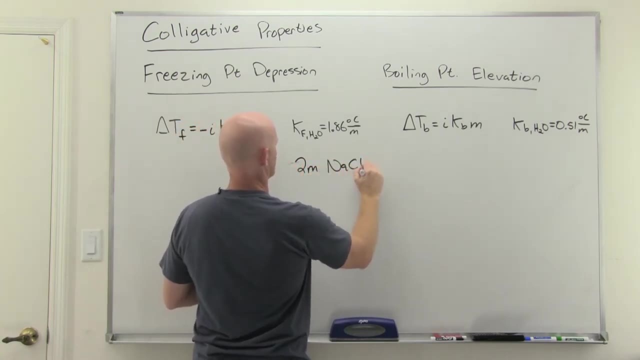 All right. So let's say I wanted to calculate the new freezing point, the new boiling point of, say, two molal. I can write the number two to make it look good: Two molal NaCl. So if we've got two molal NaCl you have to look at that and say, oh yeah, he's a strong. 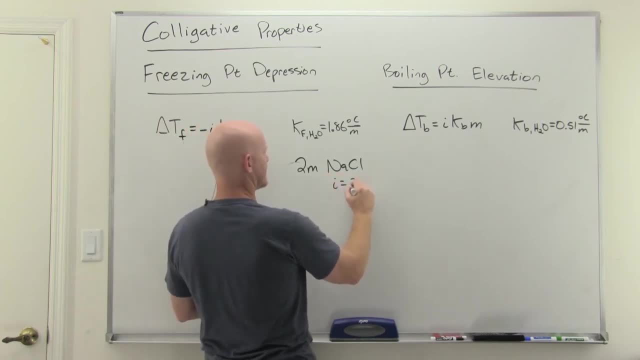 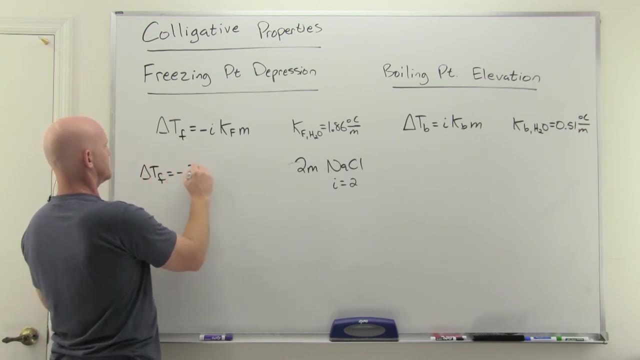 electrolyte. So you get one sodium, one chloride and your Van Hoff factor is two. OK, And from there on it's just plug and chug, And so we'll get change in our freezing point. equals negative two for the Van Hoff factor. 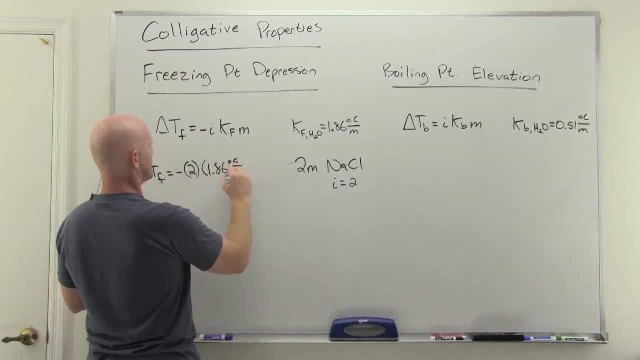 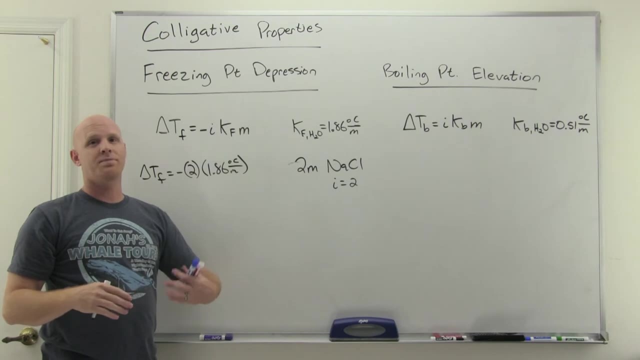 Freezing point constant here is 1.86 degrees Celsius per molal. Notice what that really means is that for every molal of total dissolved species, you get a drop in your freezing point of 1.86 degrees Celsius. Cool. And then finally, we'll multiply by our two molal constant. 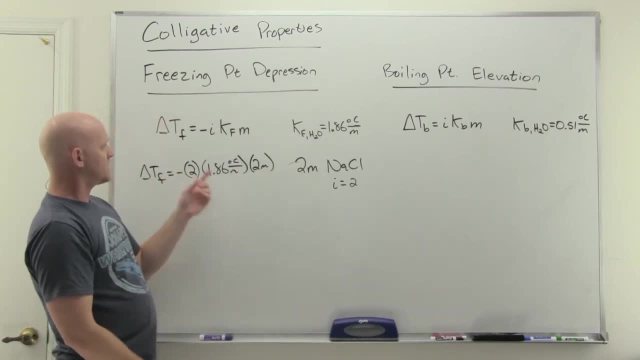 Concentration of NaCl. All right. So if you notice, by taking I times M, what you're really getting is the total concentration of dissolved species. It's two molal NaCl, But because you have one sodium, one chloride, you actually have a four molal concentration. 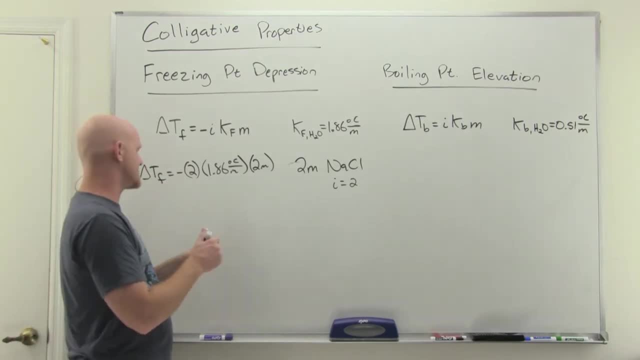 of total dissolved species And we're going to multiply that by the 1.86. And if we do so, here we're going to get negative 7.44 degrees Celsius. That is the change in our freezing point. And if the question just said: calculate the change in the freezing point, we're done. 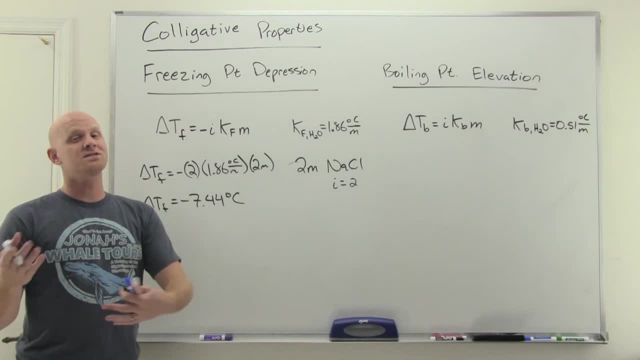 Now we're going to get negative 7.44 degrees Celsius. All right, Now, if the question said: don't calculate the change in the freezing point, but what is ultimately the freezing point? Well, your freezing point here is going to be your original freezing point, plus that. 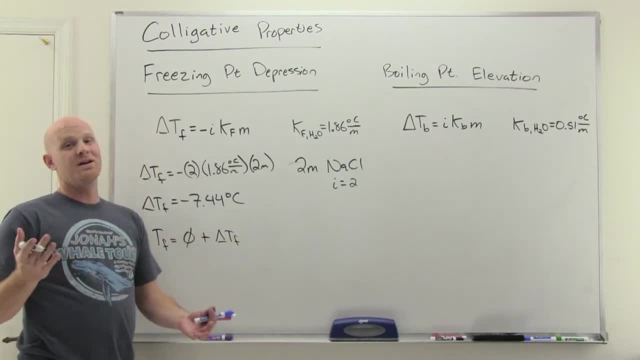 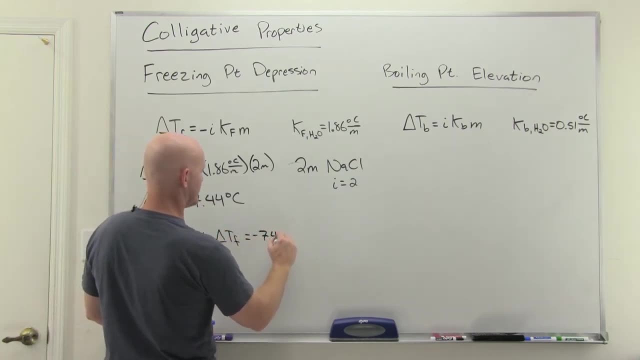 change in the freezing point. Well, it's convenient for water that the freezing point is just zero, And so when I add that change in of negative 7.44 to zero, I'm still just going to get negative 7.44 degrees Celsius. 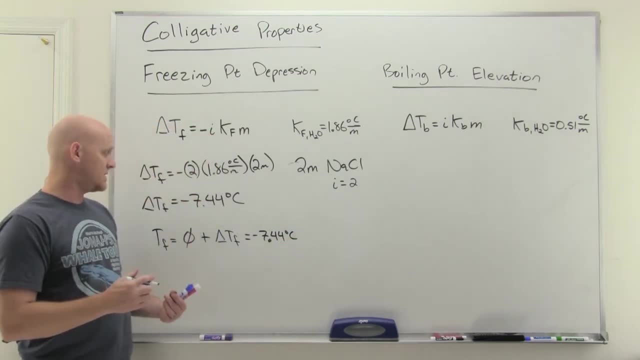 And so because water just conveniently has a freezing point of zero. so whether I say the change in the freezing point or the freezing point, it comes down to zero, All right. Well, there you go. So it comes out the same. But the reason I took pains to kind of go through the whole process here is so that 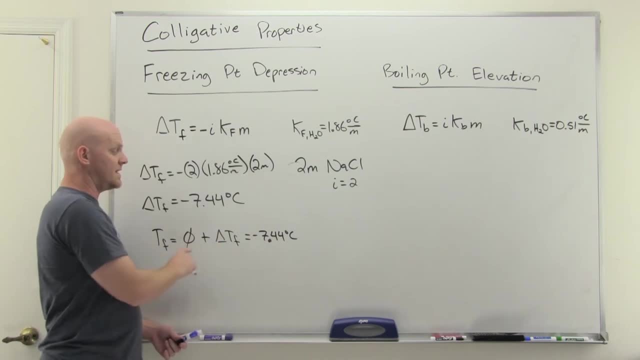 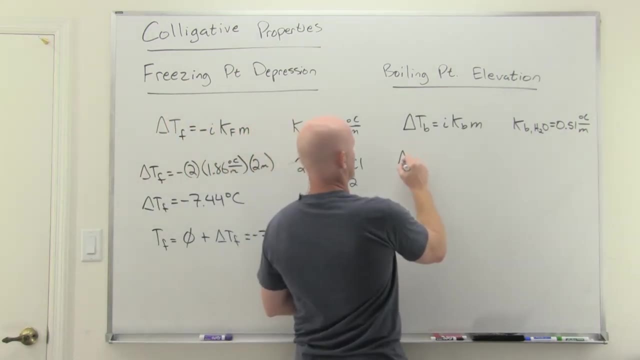 you can see that if we didn't have water, if I wanted the actual freezing point, you'd have to start with the original and then add the change to it. Now, if we do the same thing with the boiling point, here calculation works exactly the. 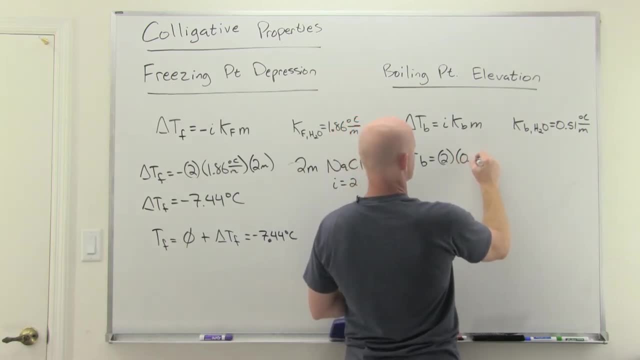 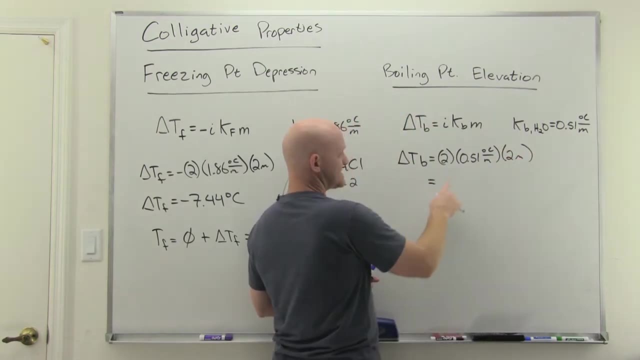 same, So two got a boiling point constant here for water, So 0.51 degrees Celsius per mole L, and again our two mole L, NaCl, And work this out. two is four, and four times a half would be two plus a little change here, so that would be like 2.04. 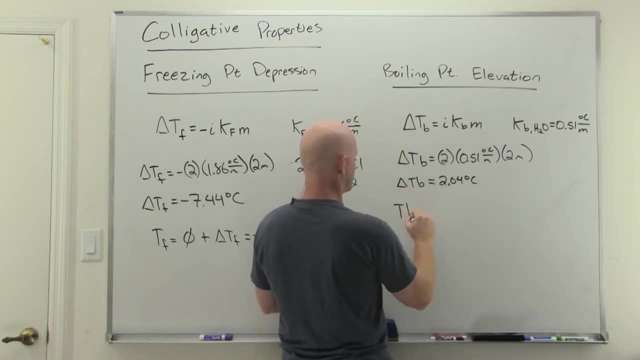 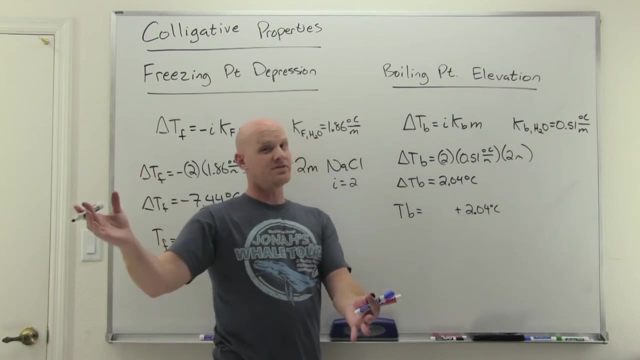 degrees celsius, and that's our change in our boiling point. now, our boiling point, though, takes the original boiling point and adds into it that change, and the original boiling point of water is not zero. in this case, it's 100 degrees celsius, and so we're going to get 102.04. 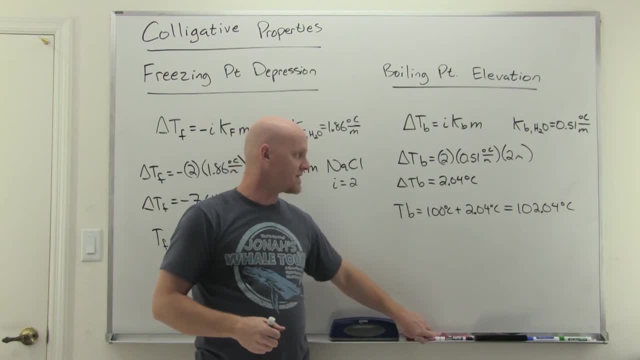 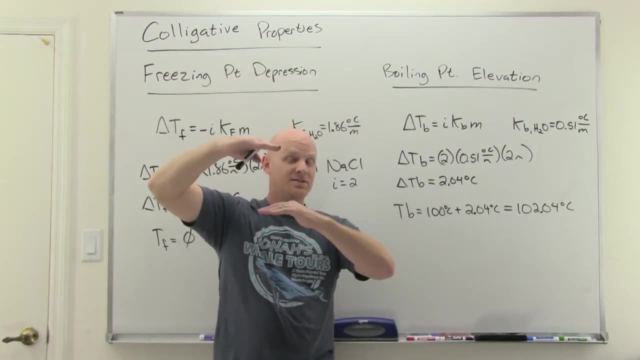 degrees celsius for our new boiling point. so you can see here that as we add solute, the boiling point goes up, the freezing point goes down and the range over which water exists as a liquid is expanded a little bit at both ends. all right, so you might have to do a little bit of calculations. 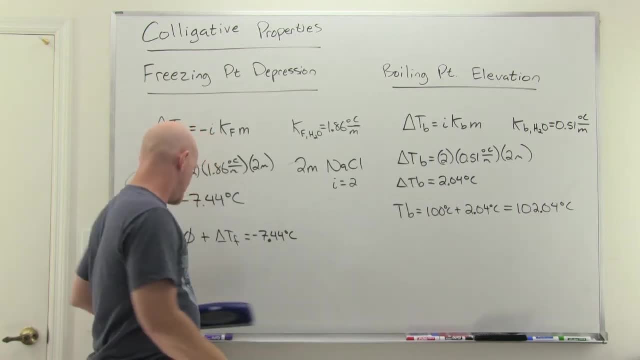 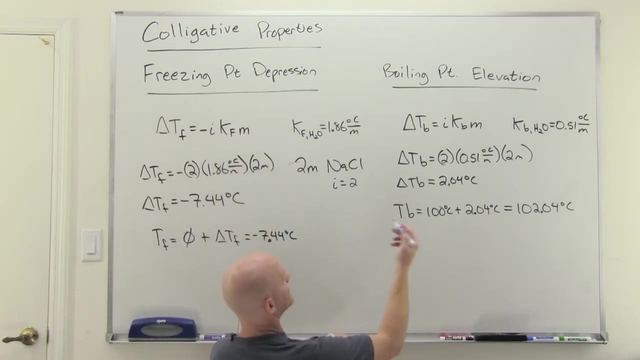 here, you know, and some plugging and chugging, you might also get a question that you can avoid doing. you know any significant amount of math on, so they might just ask you: hey, you know which of the following has the highest boiling point? for instance, and let's say i give you one, molal. 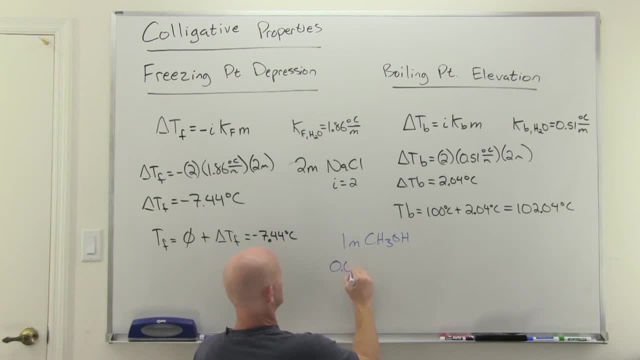 ch3oh, and i give you zero 0.6 molal nacl and i give you 0.5 molal aln033 and i give you those three solutions, as you say, which has the highest boiling point or which has the lowest freezing point or something along those. 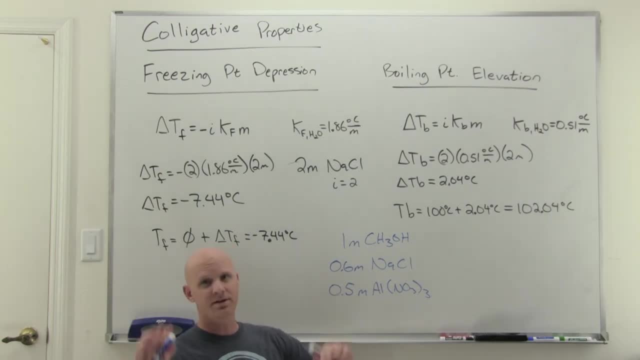 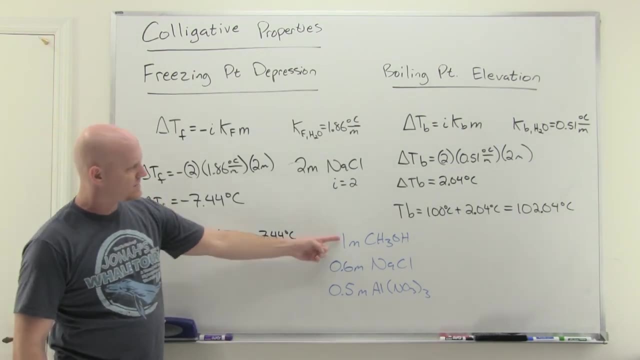 lines, and i could also say lowest boiling point and highest freezing point- same diff. but i'm going to start with highest boiling point, lowest freezing point. so in this case, what you really want to do is not just take into account the molality, but again you want the total dissolved. 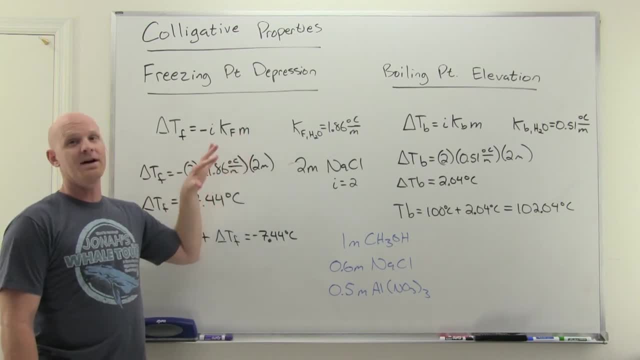 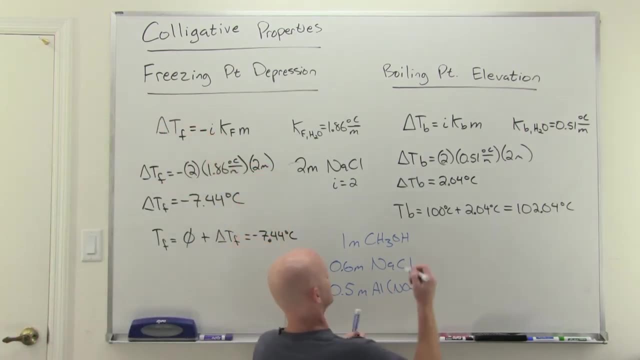 concentration which multiplies the van hof factor times the molality, and that's what ultimately is going to, you know. clue you in on this answer. so in this case, for the first one here, it's a non-electrolyte, i is one, and so i times m just equals one. so for the second one here, 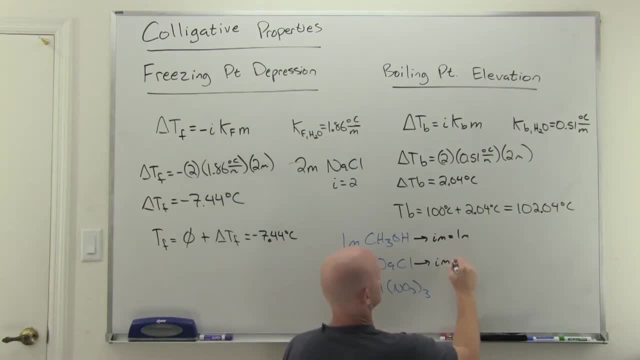 so, nacl, we said the van hof factor is two times 0.6 and you're gonna have 1.2 molal total concentration of dissolved species. so, and finally, for aluminum nitrate, we looked at him earlier, as van hof factor was four, and four times 0.5 is going to be 2.0 molal concentration of total. 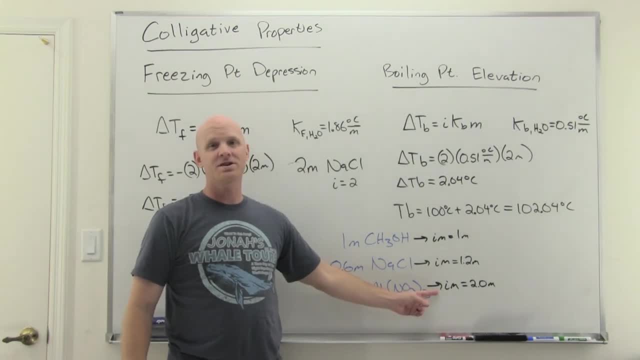 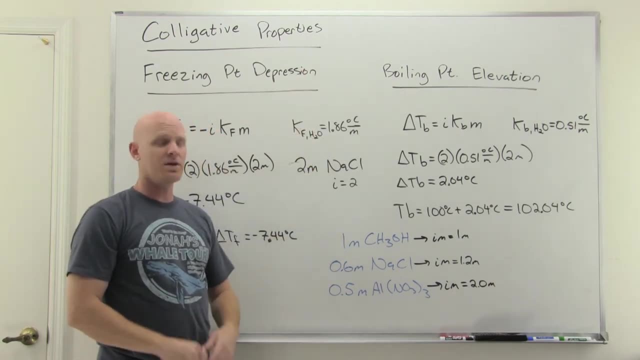 dissolved species. and because he's got the highest concentration of total dissolved species, he'll have the highest boiling point but the lowest freezing point. and so if the question was who's got the highest boiling point, aluminum nitrate wins, if it's who's got the lowest freezing point. 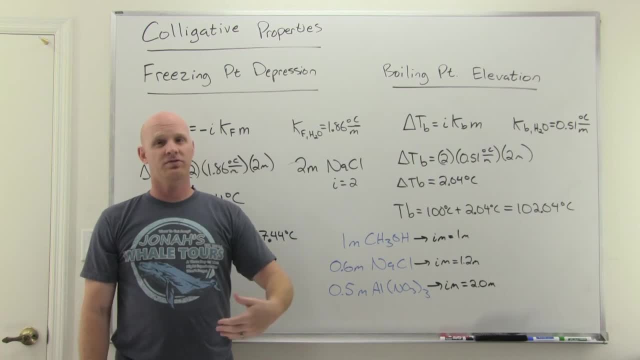 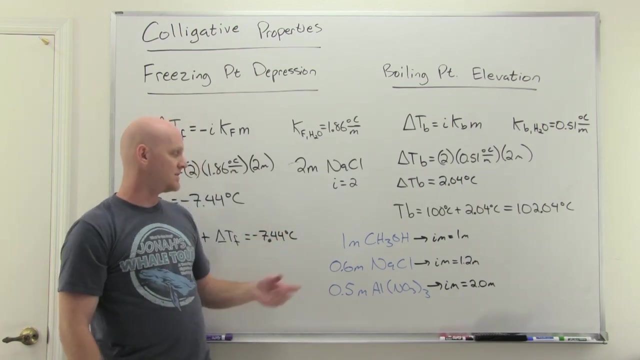 aluminum nitrate wins. however, if i said who's got the lowest boiling point, well then the one that you know goes up the least wins, he wins. but notice, the tricky one, though, is it seems backwards. but if i say who's got the highest freezing point, well, the highest freezing point is the one that has gone down the least, and that 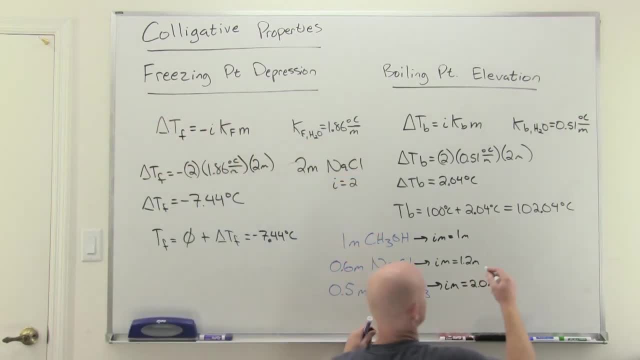 again is the methanol here, the ch3oh, and that's the one that you know students think is just the trickiest here. so but if we look at the normal freezing point for water at zero, so the methanol goes down a little, so the nacl is going to go down a little more and the aluminum nitrate is. 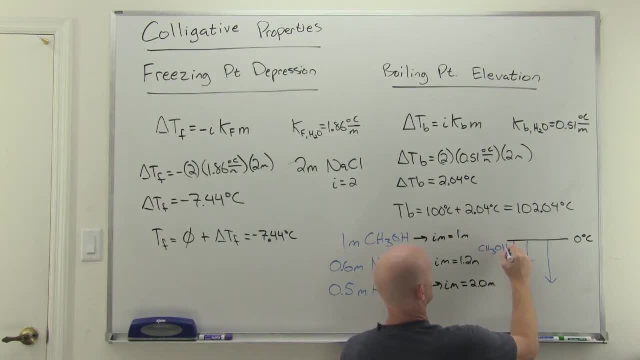 going to go down a little more yet, but the one that went down the least was the methanol, and that's why overall, kind of on an absolute scale, he's got the highest freezing point of any of those three solutions because he went down the least. all right, the next colligative property look. 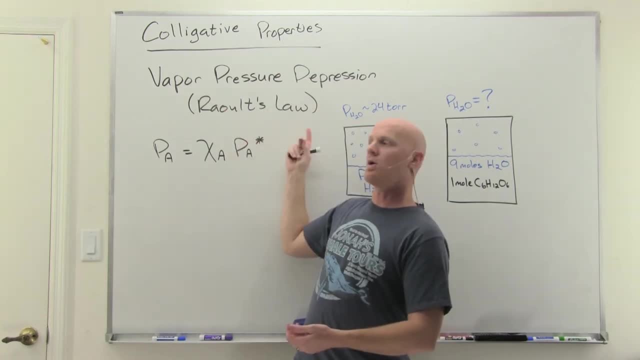 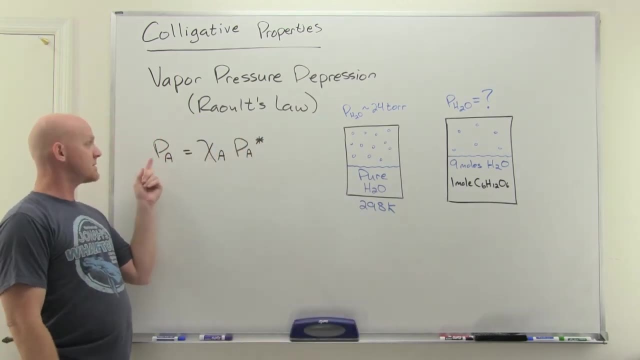 at it was it's called vapor pressure depression and it's governed by rawlitz law, which we see right here. so, and to pick apart rawlitz law real quick, so this is the partial pressure, so the vapor pressure of your solvent above a solution. this is the mole fraction of that solvent and this is the 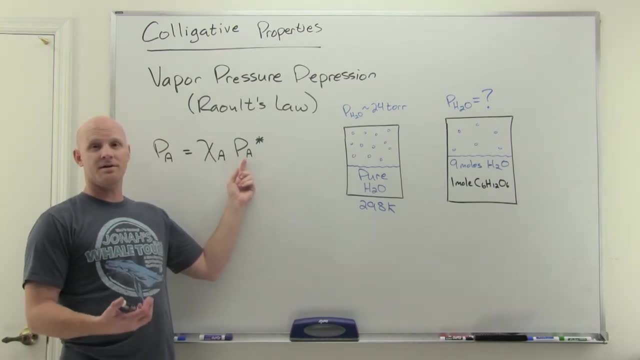 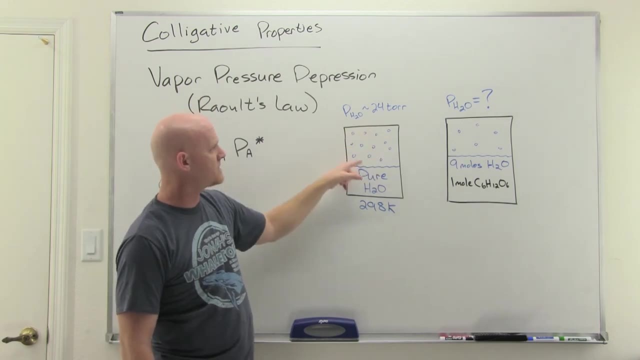 total water vapor pressure and the secret part of that solvent is that the special pressure of what your uh, or the vapor pressure uh, would be above your pure solvent in this case. so, for example, i've got pure water here and the pressure of water vapor above pure water at 298 kelvin. i'm 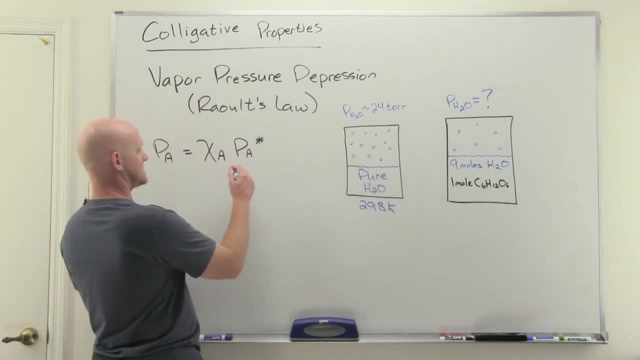 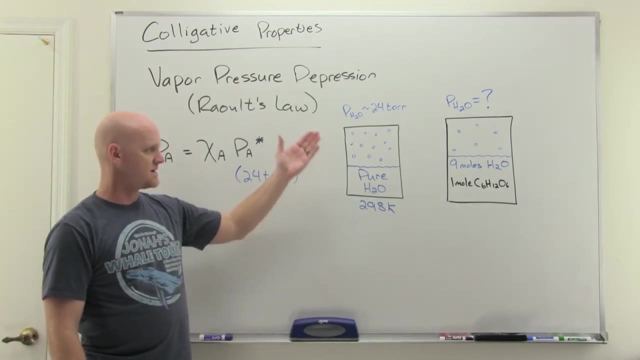 going to say- i'm going to round up- it turns out, but it's going to be right around 24 tor. so and that's what goes right here. so if you've got a solution, so in this case to know what's the vape pressure above pure water at a certain temperature, and we're going to deal. 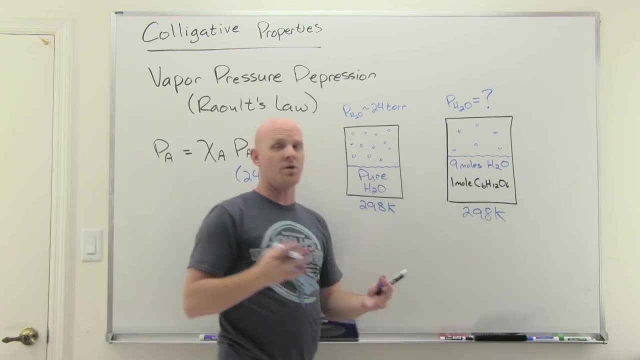 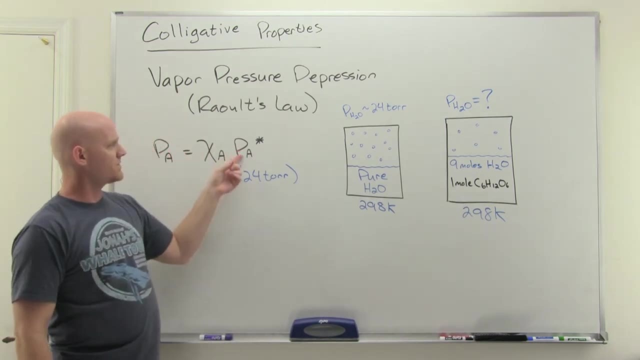 with the same temperature. so we said that vape pressure totally depended on temperature. so we have to compare, you know, pure water and a solution of water at the same temperature, so cool. so the asterisk here designates for the pure liquid. so it's 24 torr now in the second. 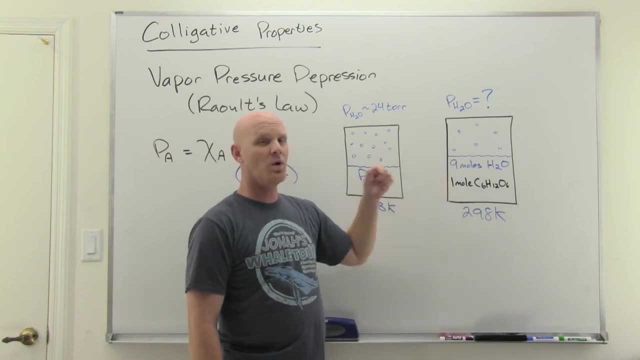 solution here. we've only got a solution that's got nine moles of water and one mole, in this case, of glucose, and i'm going to treat glucose as what we call a non-volatile solute. in this case, it's not going to have any vapor up here at all. that's what non-volatile mean. now, whether it was volatile. 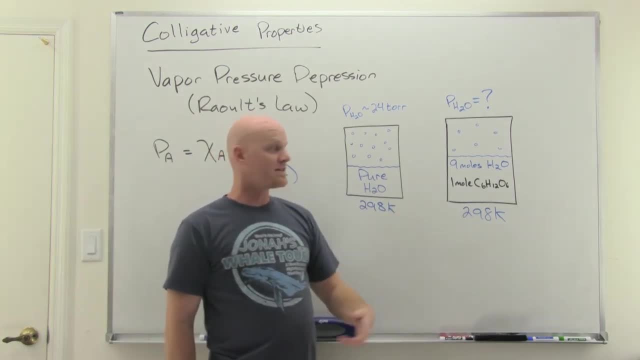 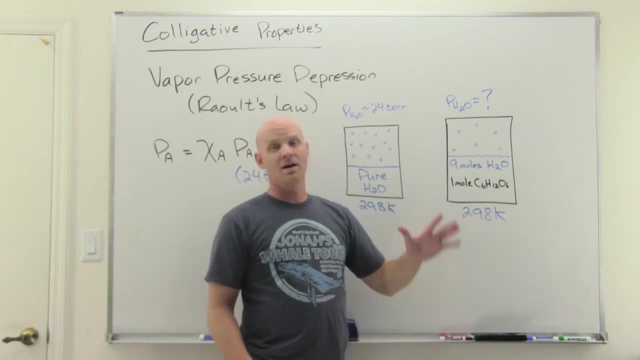 or non-volatile, it's not going to affect our calculation. but if it was volatile, in addition to water vapor up here you might have some of the solute vapor up here, like, say, i made it methanol or something that might be the case. but the calculation for the vapor pressure of the solvent 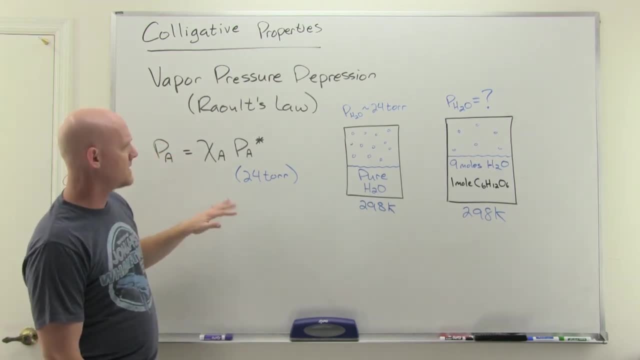 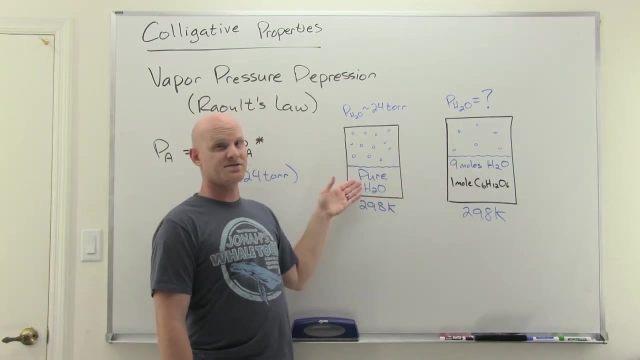 would be no different than what we're doing here. all right. so in this case, nine out of ten moles are still water. It's 90% water And because it's 90% water versus a hundred percent water, it's only going to have 90% of the vape pressure that pure water had. So if pure water has a vape pressure, 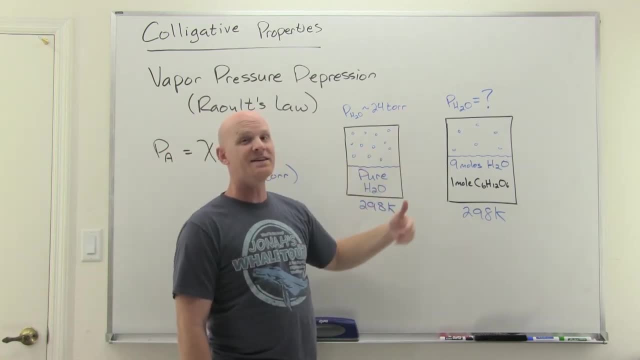 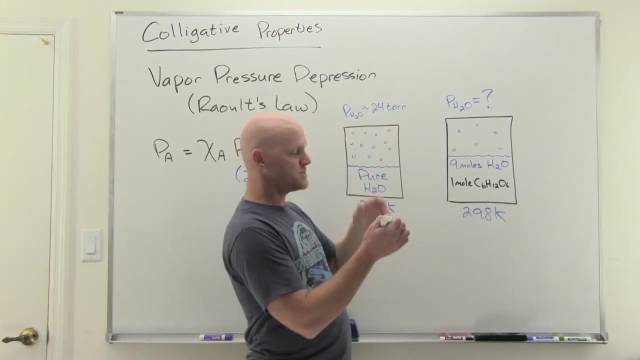 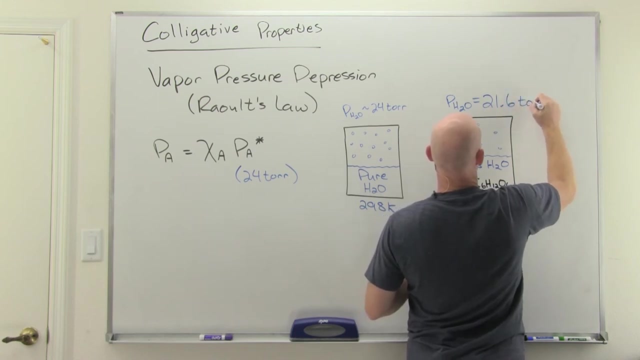 of 24 torr. so our water solution here that's only 90% water. It's only going to have 90% of 24 torr. And so if you subtract off 10%, 10% would be 2.4.. So 24 minus 2.4 is going to be 21.6 torr. 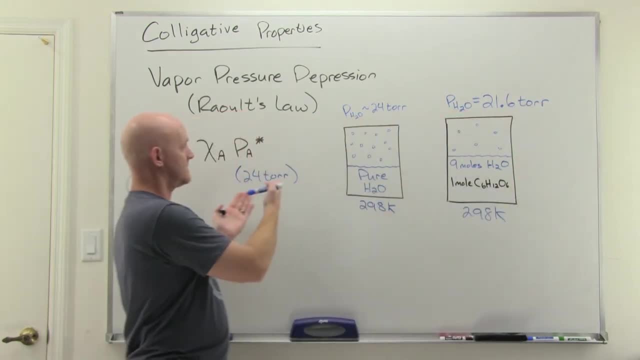 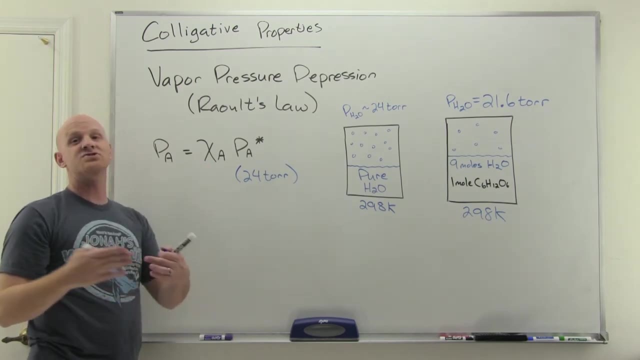 Cool And notice, we kind of did that in our heads, but I mean, we'll plug it into the equation here as well. So again this, this Greek letter chi, right here stands for mole fraction. In this case it's the mole fraction of the solvent, not the solute, And so in this case it is nine out. 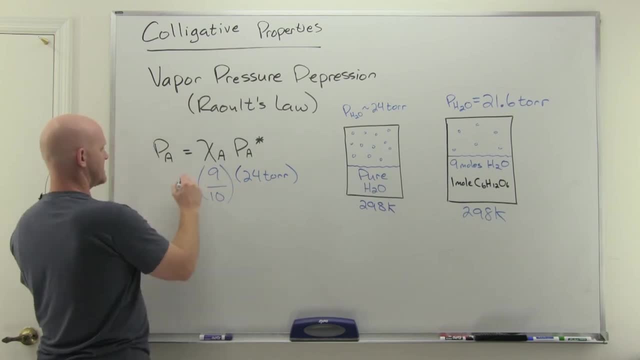 of 10.. Cool, And from there we just calculate the partial pressure of, in our case, the water. So a nine tenths of 24 torr, exactly as we already figured it out: 21.6 torr. 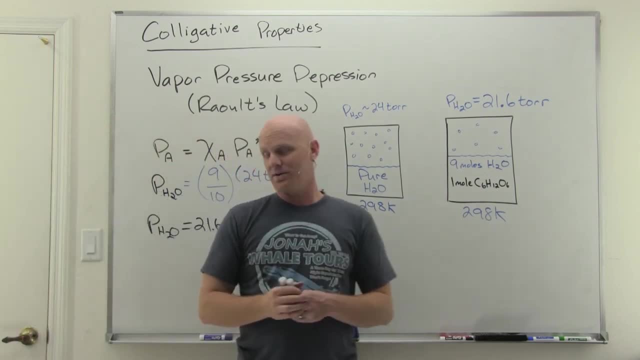 Cool, And that's really all there is to Rawlitt's law. Now it turns out Rawlitt's law is most accurate for really dilute solutions. So as you get more and more solute it gets to be less and less accurate of reality and stuff like that. So but for really dilute solutions it's a pretty. 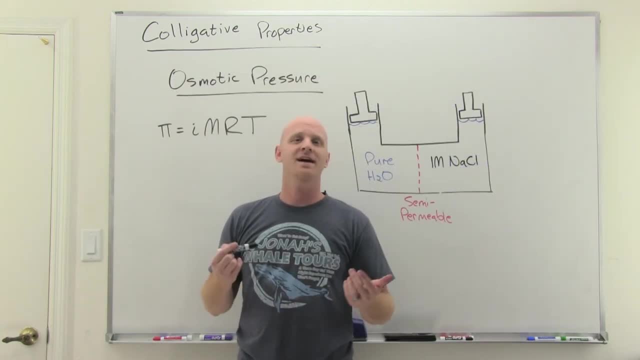 decent equation, All right. The last colligative property we're going to talk about is osmotic pressure. You might be somewhat familiar with the term osmosis, and osmosis is the diffusion of water. Now, diffusion was when something from 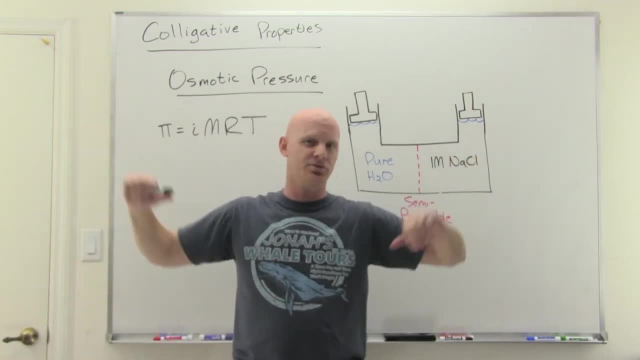 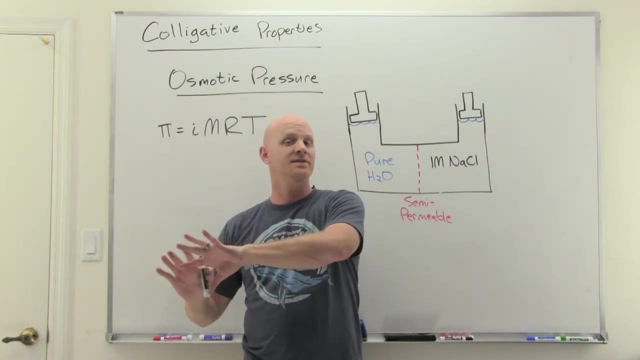 went from areas of high concentration and spread out to areas of low concentration. So, and that's what's going to happen with water here, with osmosis, where water is more pure and in a higher concentration of water, it's going to spread out and move towards areas where there's 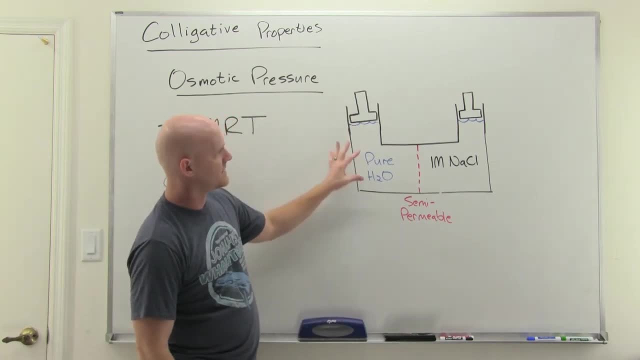 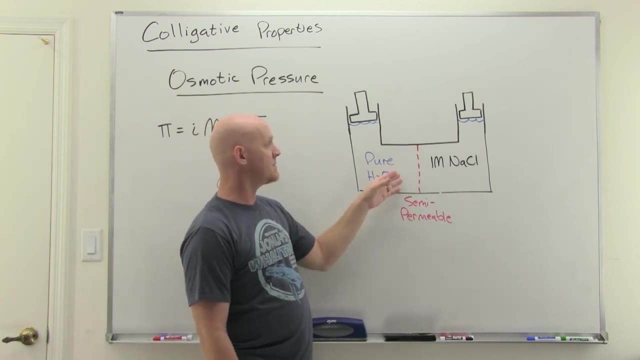 a lower concentration of water. So if we look here, we've got, like my little mock set up here and there is right down the middle of this thing a semi-permeable membrane. On the left side of that membrane there's pure water. On the right-hand side there's a one molar aqueous. 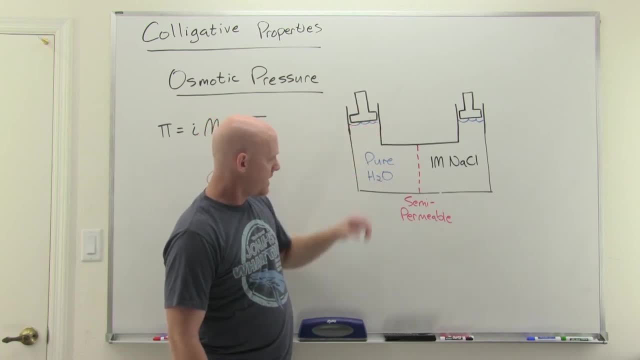 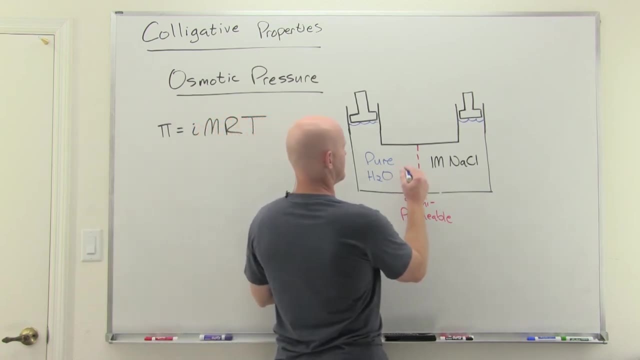 solution of sodium chloride. So and water here is more pure and in a higher concentration on the left than on the right, And so that water is going to want to travel from left to right. Now I put this membrane between the two. 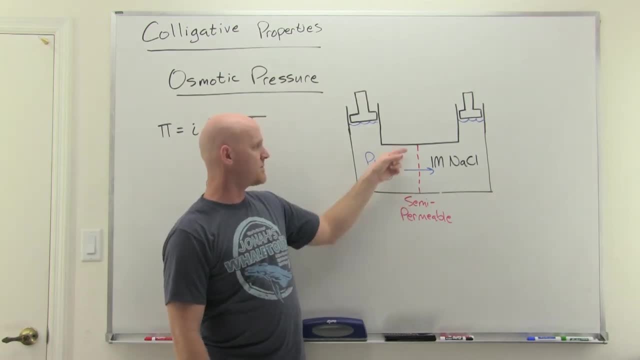 that's semi-permeable and we can select, you know, the membrane to have properties to keep, you know, allow to pass what we want to and what you know to keep in what we don't. So this semi-permeable membrane is going to allow water to pass across, but no solutes, And so in this case, 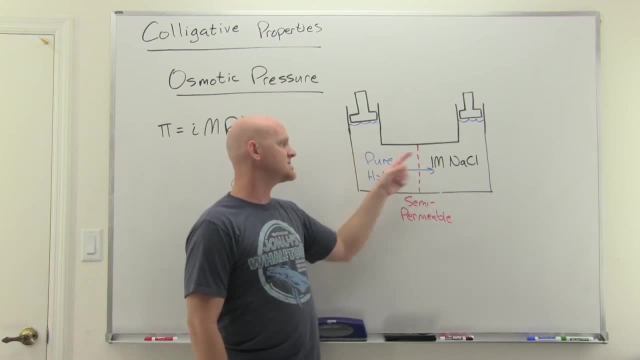 the water wants to travel to the right, from where water's in a high concentration to where water's in a lower concentration, And so that's what we're going to do here. So we're going to go ahead and select the water concentration. So the sodium chloride wants to travel left, but the membrane 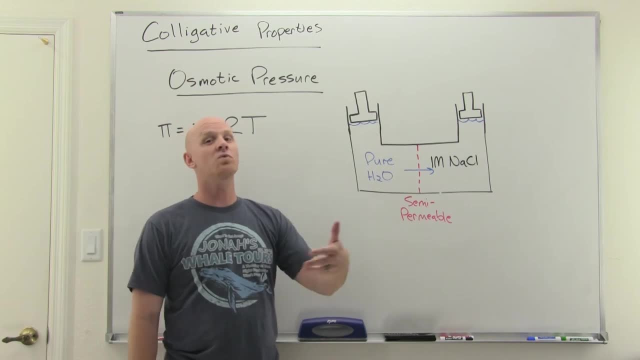 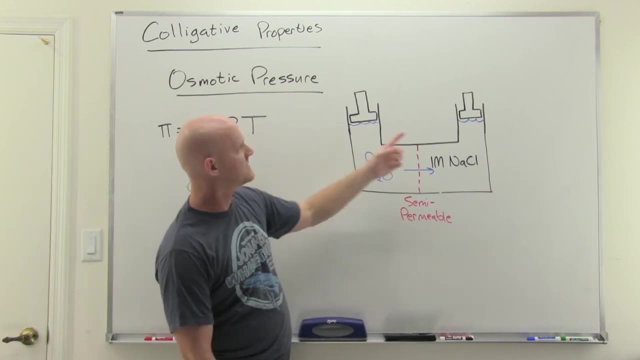 says nope, can't do it. So we only have to consider the diffusion of water, not the diffusion of solutes based on our semi-permeable membrane here. So just osmosis. As a result, you can kind of look and see on this side then what's going to want to happen to the level of the water, right? 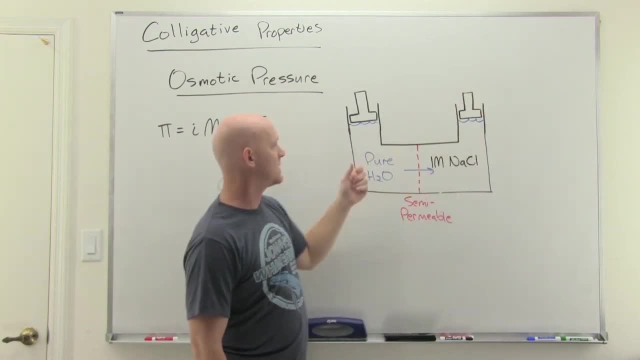 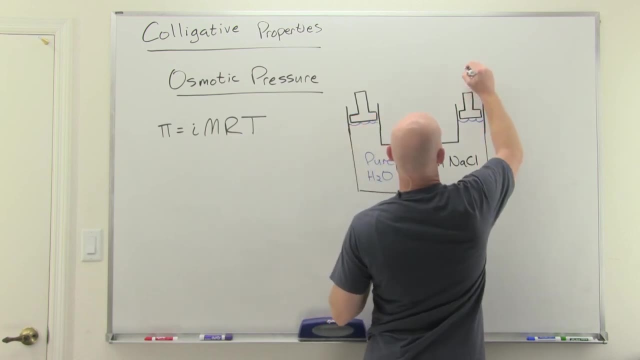 there Well, as water travels across, it's going to want to rise. And what's going to happen to the water level on this side? it's going to want to drop, And so what we're going to do is we're going to apply a downward pressure. 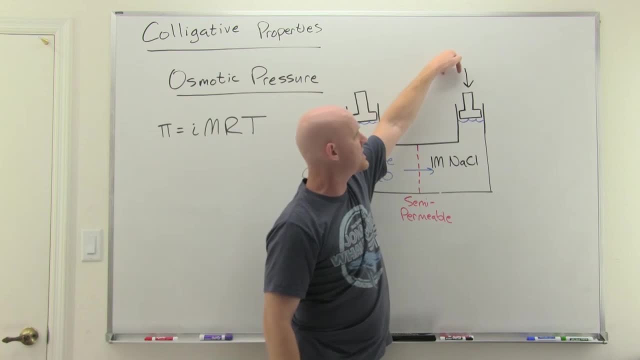 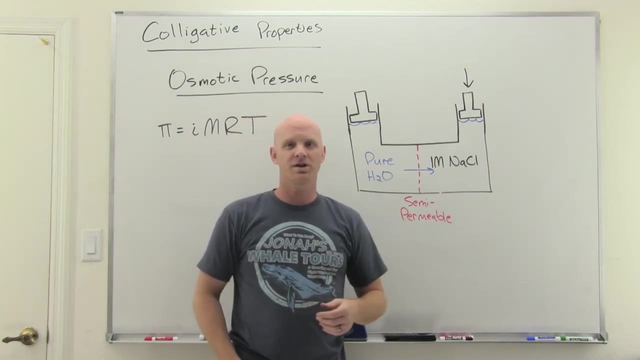 on this side And the amount of pressure we would have to push down and apply to this piston on this side to keep the water level from rising exactly is actually what's termed the osmotic pressure. So this propensity of water to want to travel this way causes a pressure over on this side. 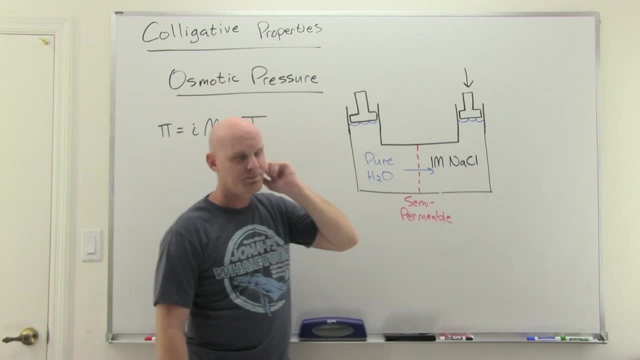 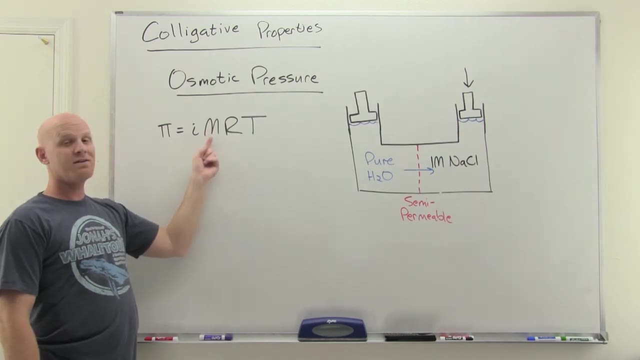 and we can counteract it right there to figure out exactly how big it is. Now it turns out the equation for it is right here. So pi equals the van Hoff factor. still factors in So times, molarity, times R, times T. So in this case with osmotic pressure, 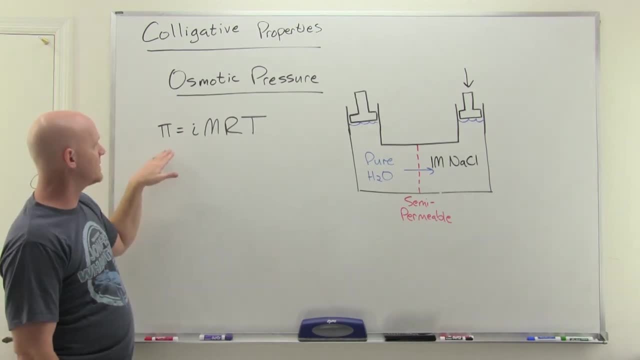 it's not molality, it's molarity. So, and also here, the Greek letter pi is what used for osmotic pressure. Now, if you recall, with our ideal gas law back in the day, we had PV equals n, RT. 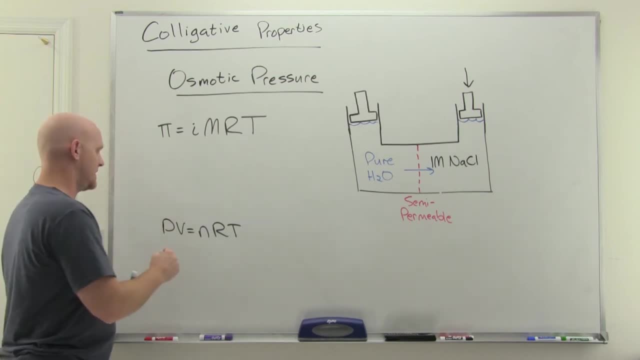 where the P here stood for gas pressure, not osmotic pressure. So, but it turns out you can kind of almost derive an expression looking like this: So just by dividing through by V, and n over V is moles over liters, which is: 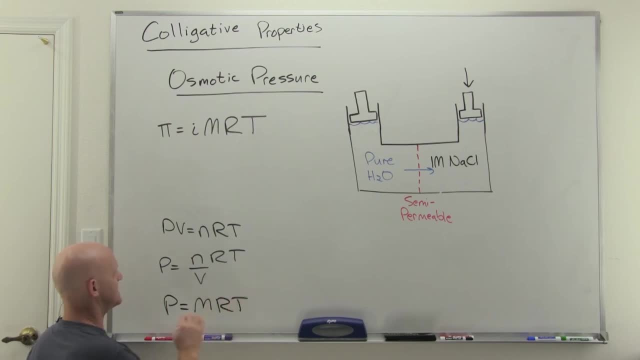 molarity And you get pressure equals molarity times RT. Now again, this is gas pressure, so it's not the same thing as osmotic pressure, But we can derive an eerily similar looking equation. Now we do have to still factor in that van Hoff factor, So, but I just want to show you. 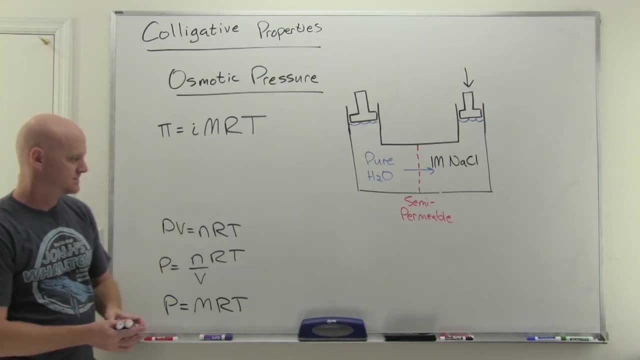 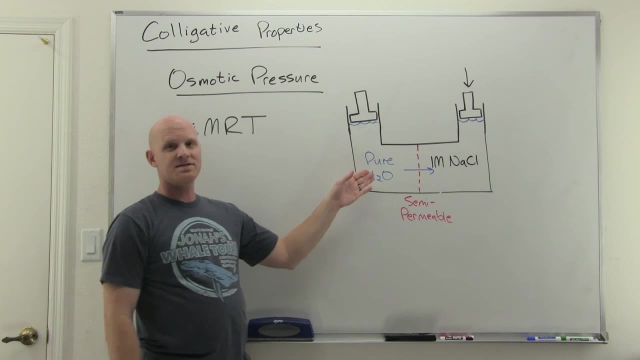 that we can kind of derive something looking similar to this from our ideal gas law. All right, so going back to osmotic pressure, So one, you're going to get things like this and you might have to predict you know which way is the water going to travel, and stuff like that. 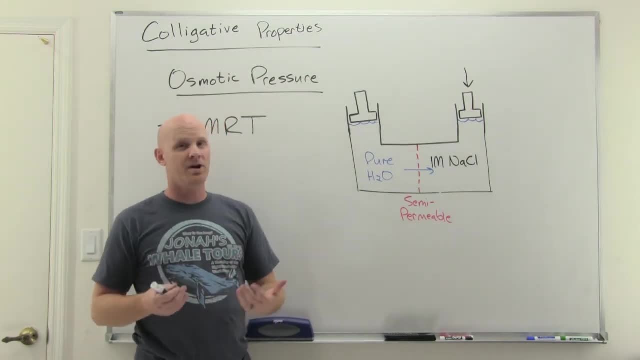 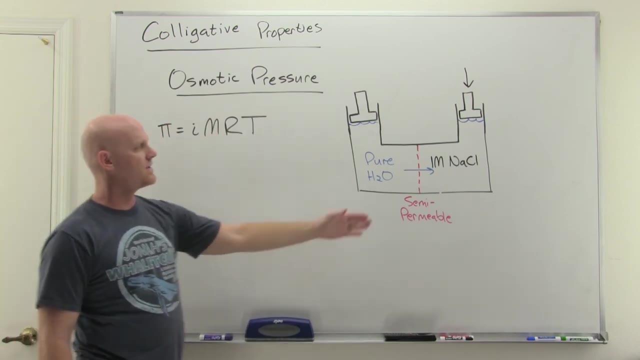 Or you might have to look and predict. you know where you're going to have greater osmotic pressure and things of that sort. So if you look at the way this works in our calculation here, so pi equals IMRT. So in our case the NaCl is our solute. 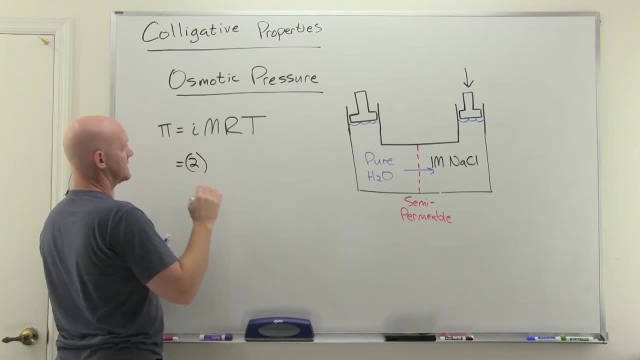 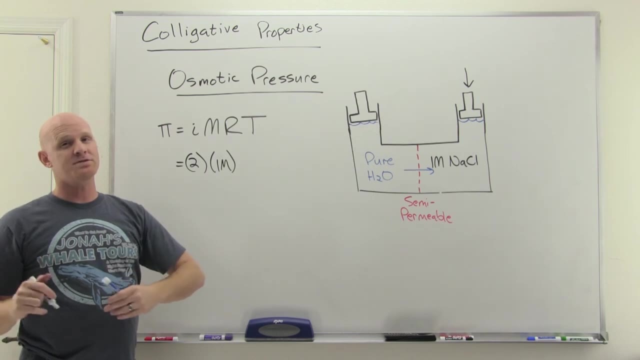 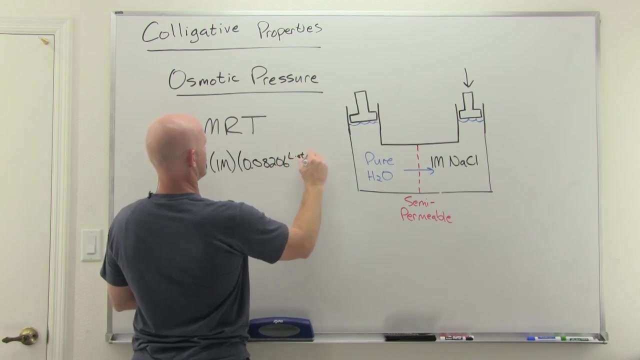 it is a van Hoff factor still of two. the molarity of it was one molar, So R here. so we want to come out with units of pressure, And so I want to come out in atmospheres in this case. So I'm going to use our classic value of R of 0.08206 liter atmospheres per mole Kelvin. 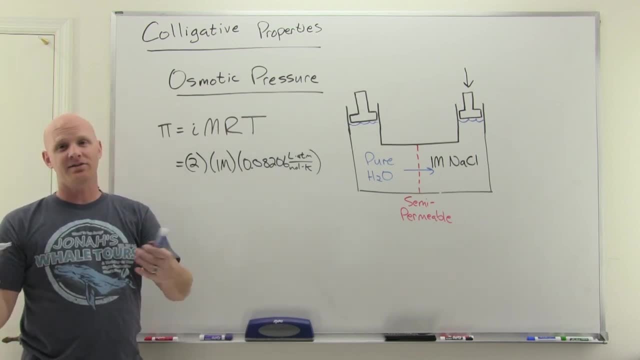 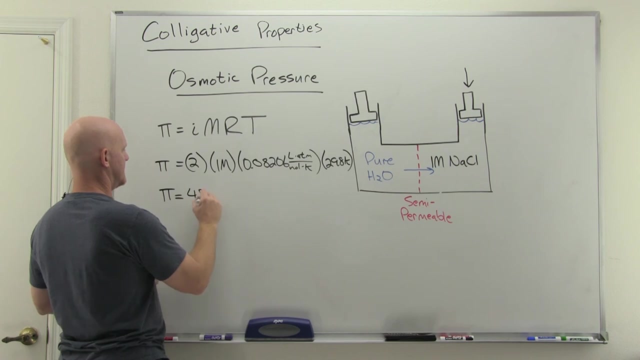 Cool. And then I want to calculate the osmotic pressure specifically at 298 Kelvin. So that has to be given as well. Cool, And from there it is plug and chug. So, and if we work this out- and conveniently I already worked it out- So with my handy dandy calculator, it's 48.9. 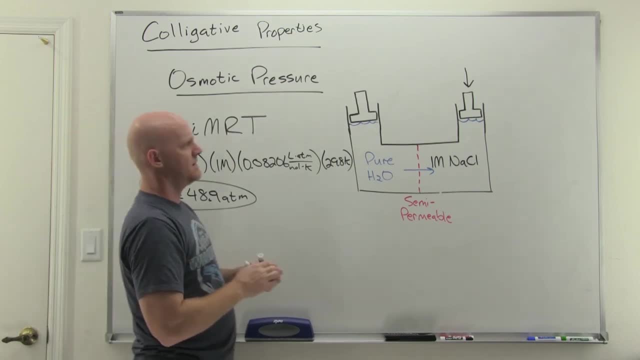 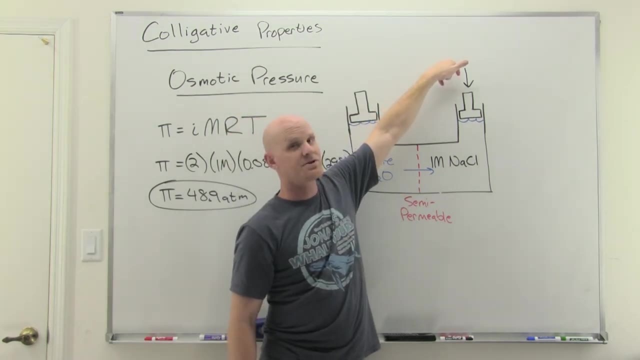 atmospheres. that would be the osmotic pressure So being exerted as the water tries to travel from the left hand side to the right hand compartment. So if you pushed down here a pressure of exactly 48.9 atmospheres, you would keep the water level from rising Now. 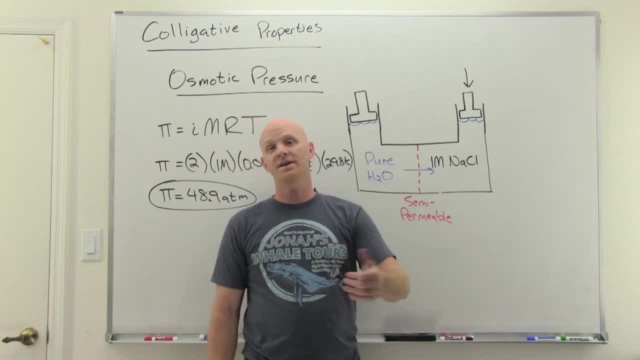 what would happen if you only pressed with a pressure of 40 atmospheres? Well then, the water level is going to rise. So what if, on the other hand, you pressed with a pressure of 100 atmospheres? Well again, the osmotic pressure is only exerting an upward pressure. 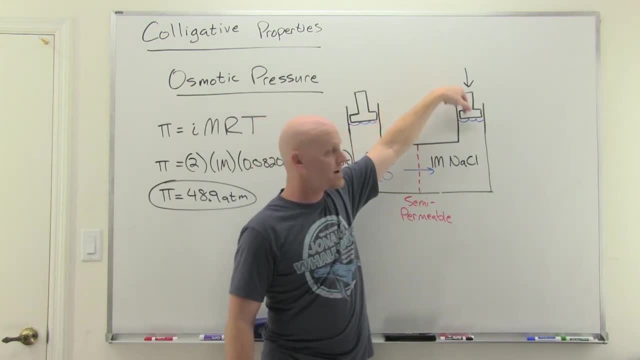 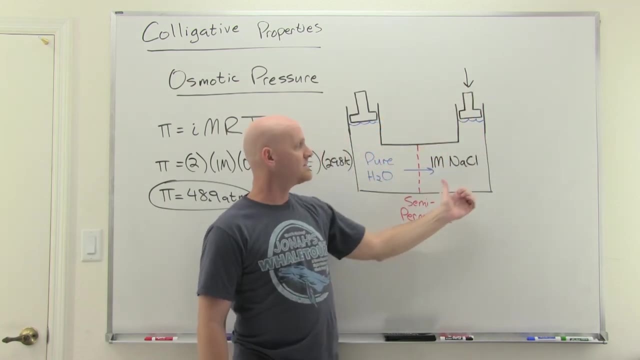 of 48.9 atmospheres. If you press down and apply a pressure of 100 atmospheres, you win and you're going to actually cause the water level to decrease. you're going to push that piston down And that's going to force water to the other side of the semipermeable membrane And 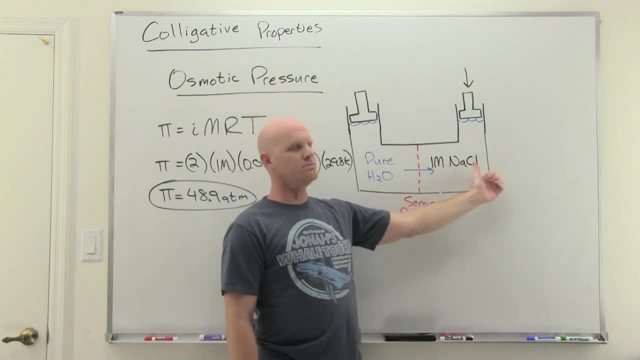 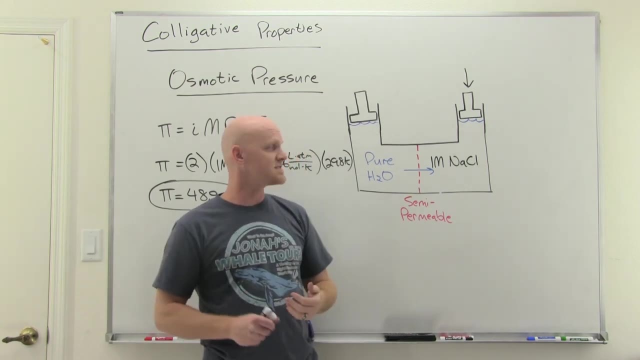 you're going to make more purified water. So you're actually causing osmosis to go in reverse and make purified water. That sounds familiar. You're doing reverse osmosis. That's how a reverse osmosis system works. So big problem, though, here is that initially you're pushing down with 100. 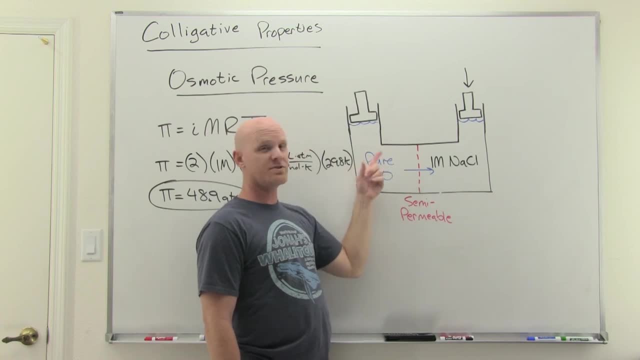 atmospheres. But notice what happens here: As you force water across to the other side, the concentration of salt over here. It's actually going to increase as you get rid of more and more solvent, more and more water to the other side, And as that increases, then your osmotic pressure goes up and eventually you'll